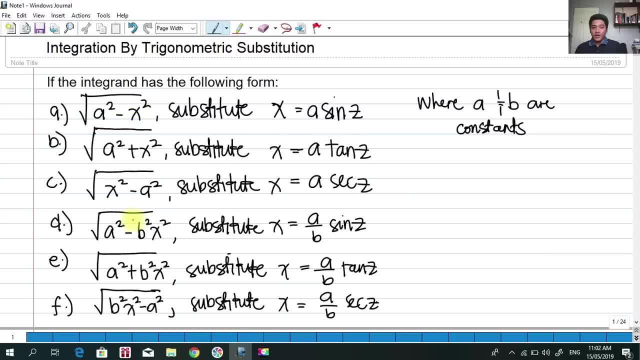 now of x squared is not already one. okay, So we can substitute: x is equal to a secant z here. because b is another constant, we can substitute x is equal to a over b sine z. okay, Again, this is only a, this is only b sine z. So, as you can see, this is a general form. 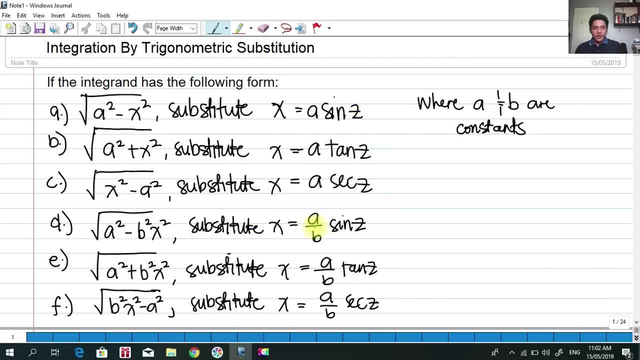 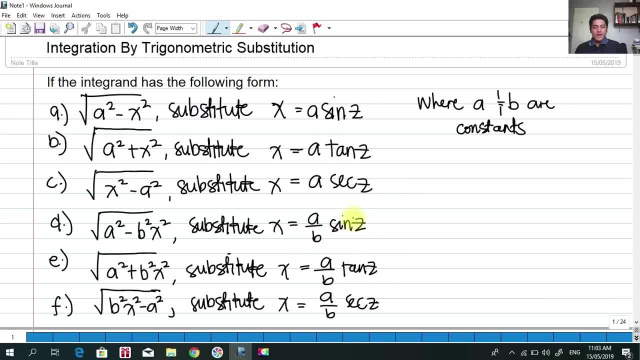 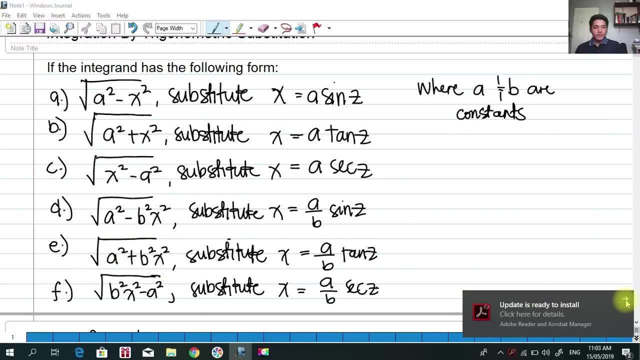 of the first is actually this: okay, So it so happened that the coefficient of this is one, so a over one is simply a sine z. okay. So for letter e, we have the square root of a squared plus b squared, x squared. okay, We can substitute: x is equal to a over b, tangent z and again. 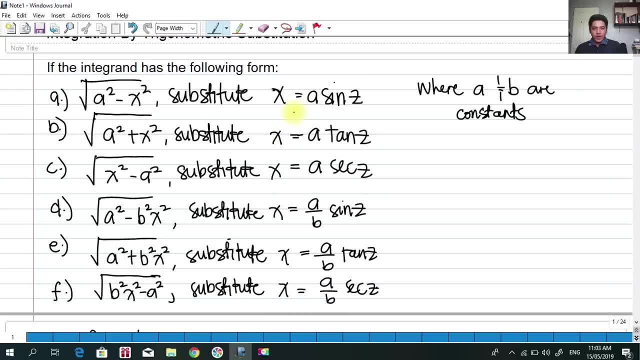 this is a general form of our letter b formula. okay, We're again. we can substitute: x is equal to a over b tangent z, and again, this is a general form of our letter b formula. okay, We're again. 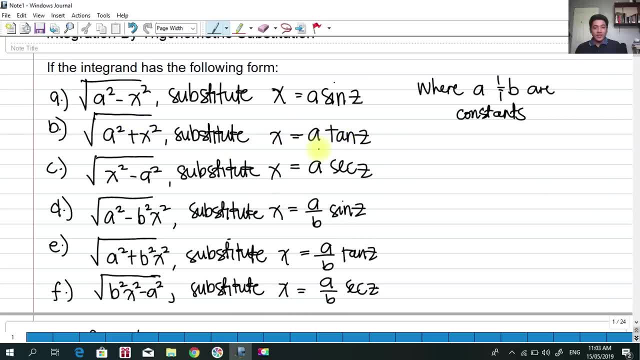 the coefficient here is one, so a over one is simply a tangent z. but if the coefficient is not one but rather greater than one, we need to use this formula. okay, And another. for the last one, we have the square root of b squared x squared minus a, squared that is equivalent to x is. 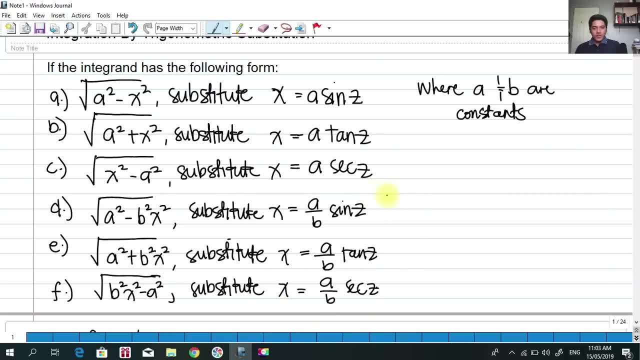 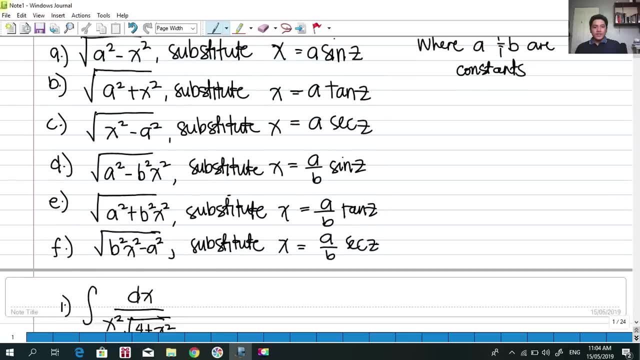 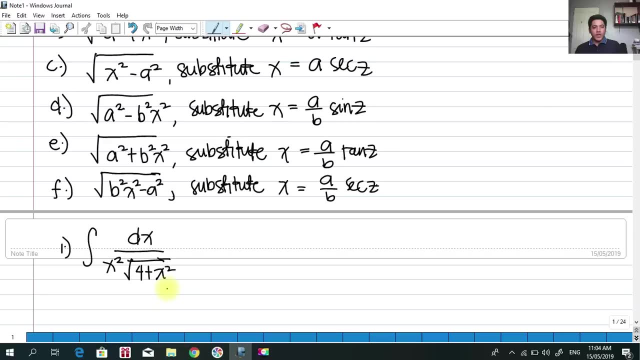 equal to a over b, z. Again, this is the general format of our expression. okay, So let's try to solve this problem. So, let's try to solve this problem. So let's try to solve this problem. For number one, we have the integral of dx over x squared times the square root of 4 plus x squared. 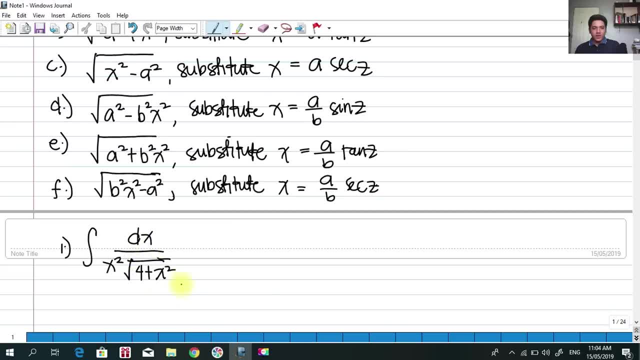 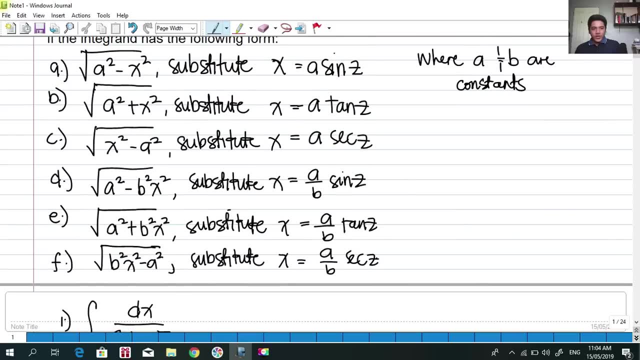 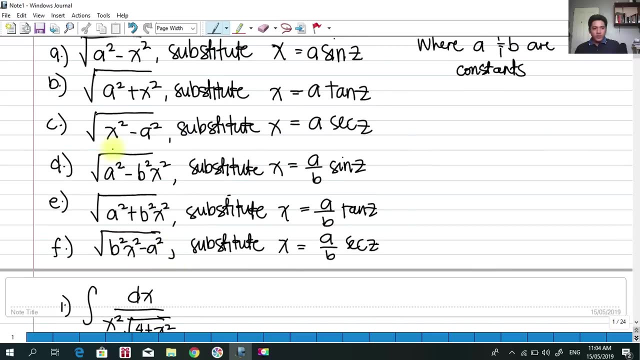 So what are we going to do is to identify first the integral. The integral has this following format: square root of 4 plus x, squared. If we're going to look at our formulas here: square root of 4 plus x, squared plus. so the coefficient of x squared is one. so these three, d, e, f- we cannot use. that, okay, But rather we can use: 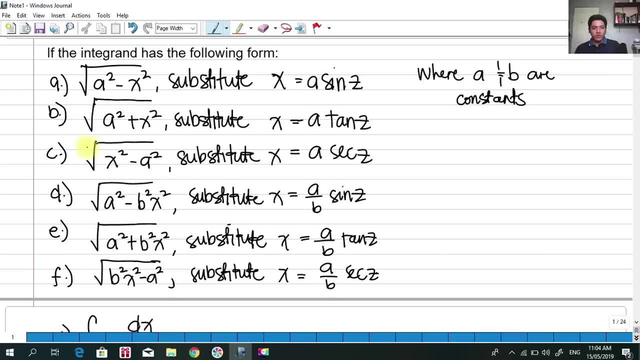 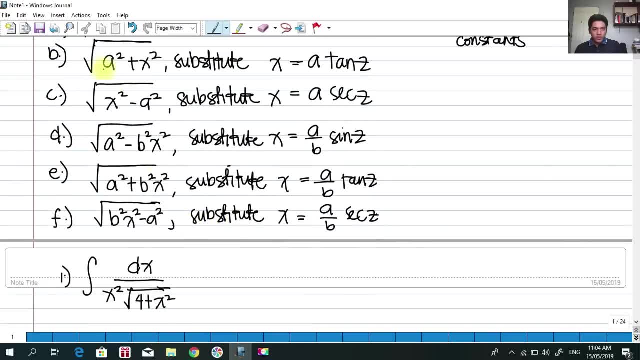 the letter b formula, wherein it has a form of square root of a squared plus x squared. then we're going to substitute: x is equal to a tangent z. So this has a form of square root of a squared plus x squared. okay, So now what are we going to do? is we're going to simply what Let: x is equal to a. 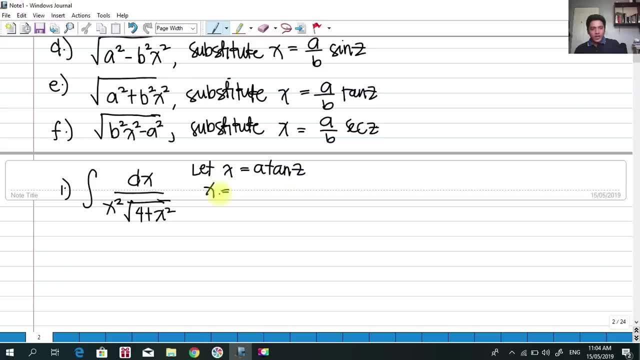 tangent z, where our x or a. here is this: four. take note that this is already squared, so that is a squared. To get a, we could get the square root, that is a 2 tangent z. This is very important. this equation is very important because you have to. 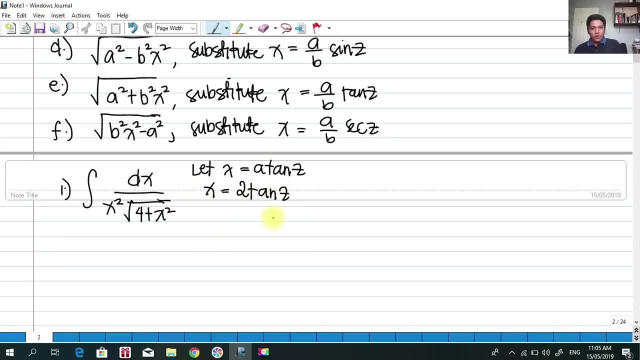 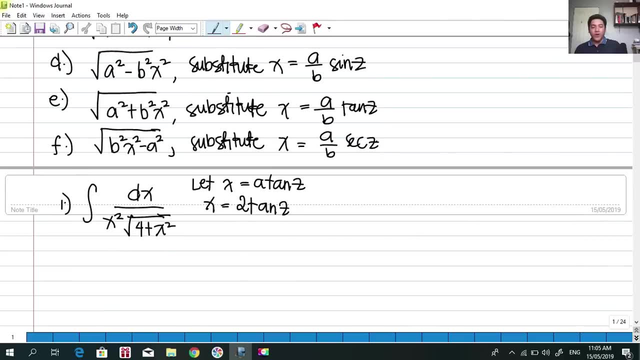 from this equation we can derive the triangle. okay, So, by the way, in this integration by trigonometric substitution, we're going to use a right triangle in solving this integral. okay, So we can. how can we write the right? 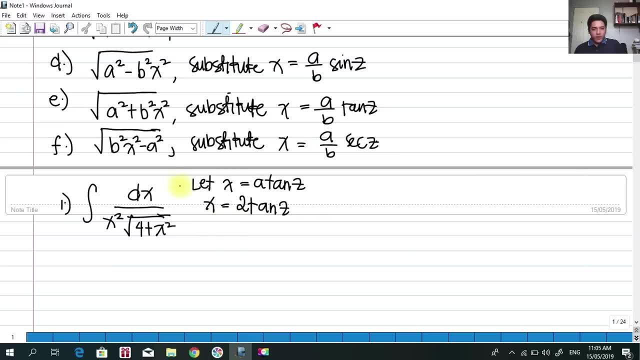 triangle. It's based on this equation. So from we can get tangent z, okay, We can isolate tangent z, and that is basically x over 2.. And if we're going to create a triangle, a small triangle here, a right triangle, okay, Wherein this is the hypotenuse and this is an angle we call that. 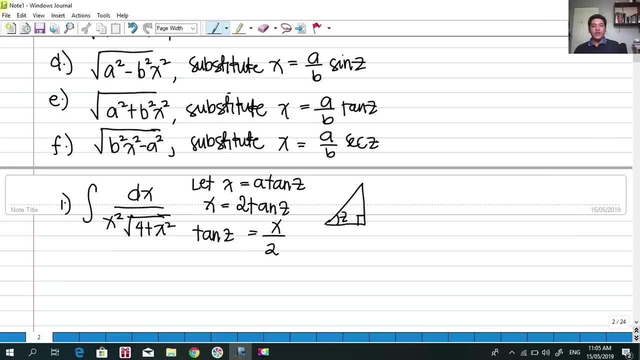 by convention, the angle z or this z. okay, So from this relationship tangent z- z is equal to x over 2.. So for a right triangle we can actually assign this on the sides of the triangle by what we call the isokatawa. okay, Tangent z is tawa, so it means opposite over adjacent. 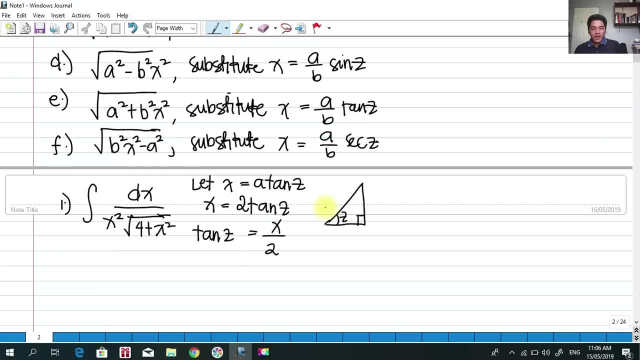 So this is the z. okay, This is the z angle, so its opposite is this side. so this must be the x and its adjacent side is 2.. And therefore, if you're going to get by Pythagorean theorem, the hypotenuse, that is 4 plus x squared, of which this is now. 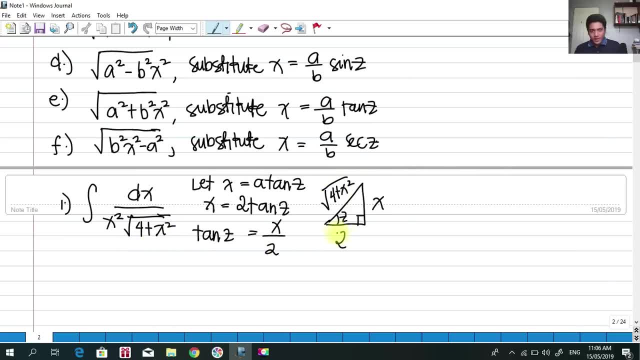 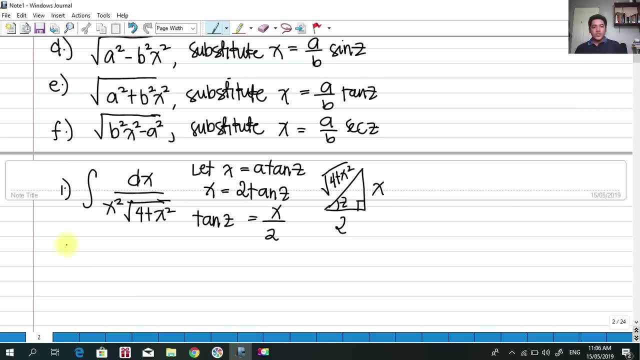 our integrand here. okay, This is very important. okay, So as to know what will be the size of your triangle. okay, Well, of course, trigonometric substitution. we already got the x, So we have, we can get, we can substitute it here: x squared by simply squaring this. But the problem is we 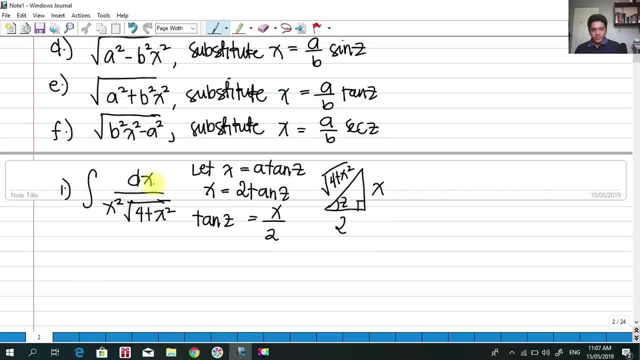 still need to get the x squared, So we can substitute it here- x squared- by simply squaring this. But the problem is we still need to get the x squared, So we can substitute it here: x squared by d, x and the square root of 4 plus x squared, So we can get the x by simply differentiating this. 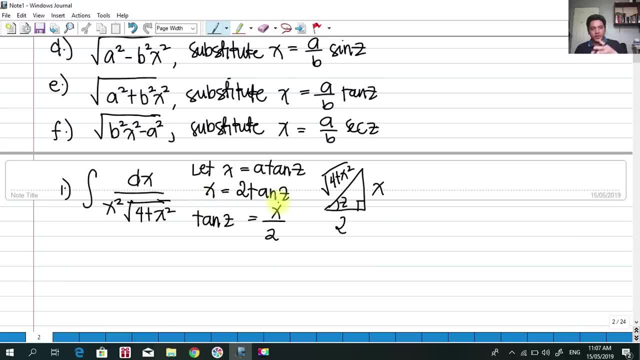 both sides, So differentiating it to the left with respect to x and differentiating this with respect to z. So if we get the derivative of x is equal to 2 tangent z. that was b. dx is equal to what 2 secant squared z with respect to z. so we have to include d? z. So we get now the dx and how we. 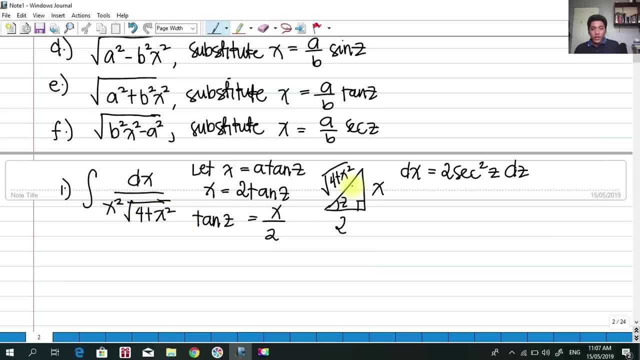 are we going to get the square root of 4 plus x squared Well by looking at this triangle? okay, So as much as possible, we want to try to avoid this side which has an x. okay, So we're going to. 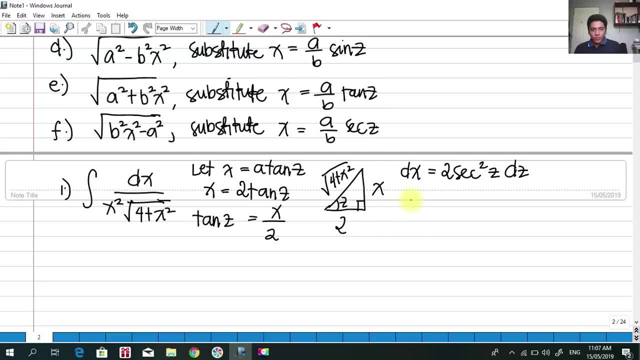 try to avoid this using this side. okay, with respect to z. okay, So in avoiding this, we cannot use sine because sine has an opposite. We cannot use also cosecant because it has an opposite. okay, So we can use cosine, cosine of j. Cosine of j is adjacent over hypotenuse. But if you're going to 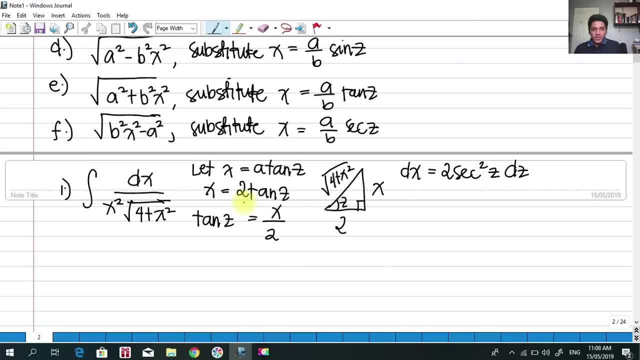 look at our x and dx, it is in terms of tangent, in terms of secant. So we can use the secant function How? By reciprocating the cosine, because 1 over cosine is secant. and if we reciprocate that, instead of objecting the cosine, we can use the secant function because it can also be a. 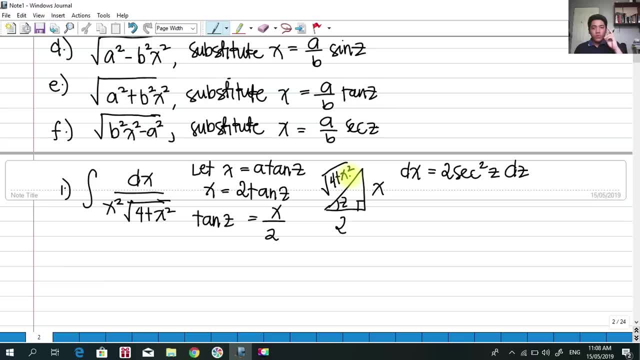 Adjacent over hypotenuse for a cosine. so secant z now will be what? Hypotenuse over adjacent. So hypotenuse will be 4, square root of 4 plus x squared okay, over 2.. And if we're going to get square root of 4 plus x squared, 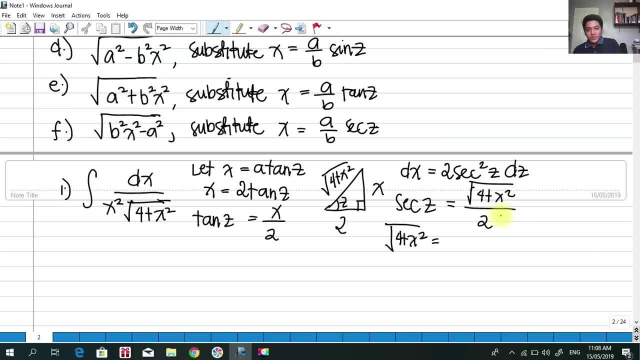 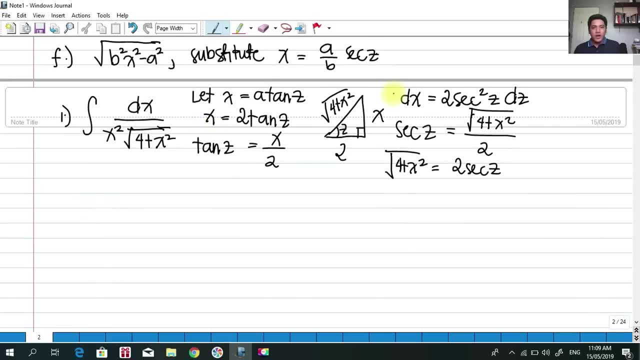 because that's what we are after- to make a substitution that is 2 secant z. Okay, we're done here. So we have the x, we have the dx and we have d squared of 4 plus x squared, So we can substitute it to our integral now. 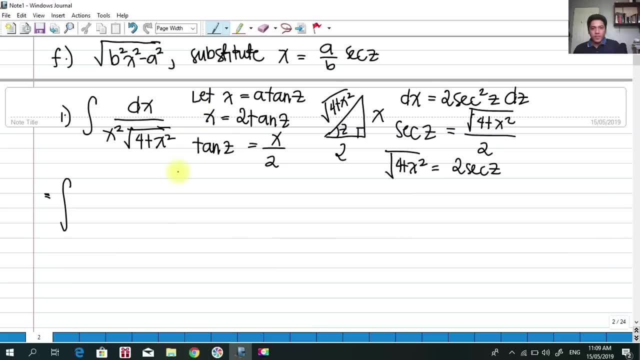 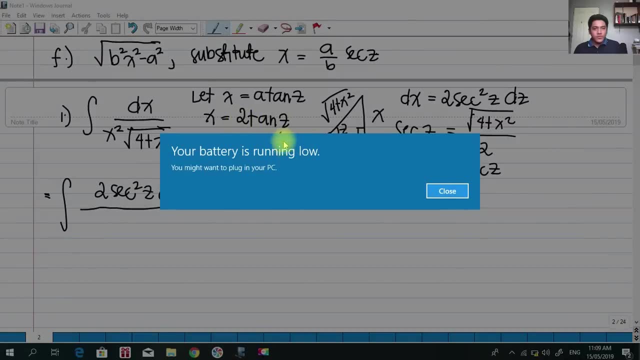 Our integral will now be: dx is simply what: 2 secant squared z dz. So 2 secant squared z dz over x squared. So we have to square this. We have to square this side. okay, We have to square this side. 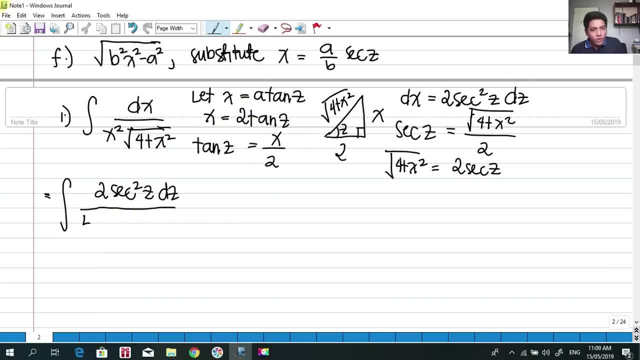 And upon squaring that so 4, that would become 4 tangent squared z multiplied by the square root of 4 plus x squared, which is actually 2 secant z. So 2 secant z. So what will happen is that, by simplifying our integral, 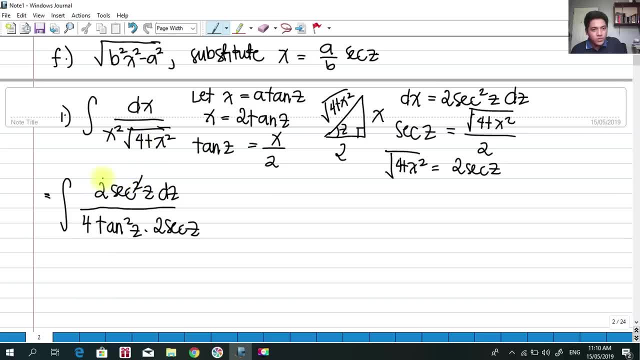 we could cancel out this 1 secant, 2 secant here and also of course, the 2,. okay, And 2 secant here will be canceled also. okay. So cancel, cancel. So we are left with secant z. 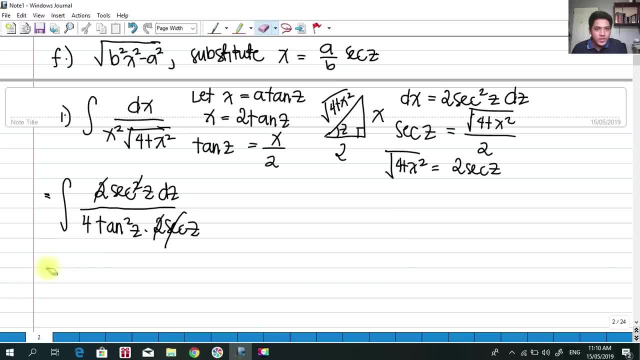 So let me just rewrite it here so that you can see it. We can save some space. So that's the integral of what Secant of z, dz over 4, tangent squared z. So we can factor out 1, fourth outside of the integral. 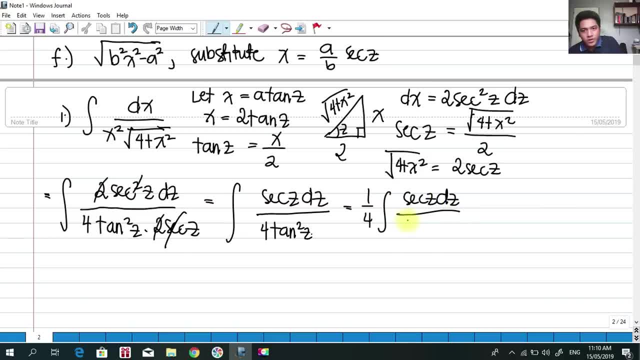 and we are left with secant z, dz over tangent squared z. And if we can simplify that, 1, fourth, the integral secant z is 1 over cosine z by reciprocal identity and tangent squared z is simply sine squared z over cosine squared z. 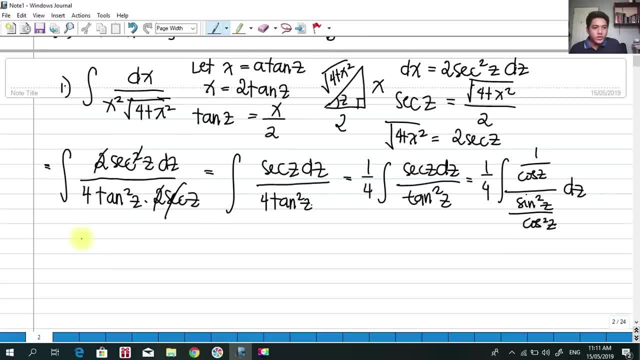 And that is basically still dz. So if we're going to get the reciprocal of the denominator and perform multiplication, we can get what 1 over cosine of z multiplied by cosine squared z over sine squared z, dz. And as you can see here, 1 cosine here will cancel. 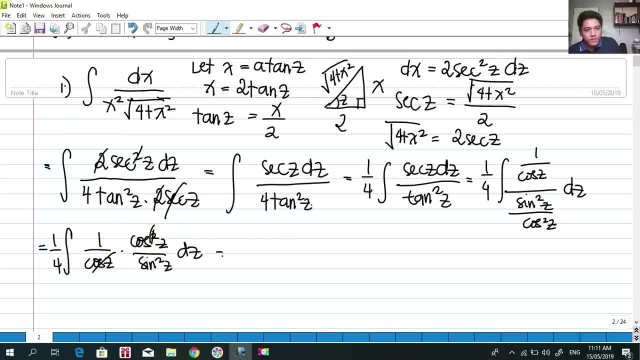 So this would be canceled. So we are left with 1 fourth integral of cosine of z over sine squared z, dz, And this will be very pretty much for a straightforward integral If we're going to rearrange this. so we have 1 fourth integral of sine z raised to negative 2.. 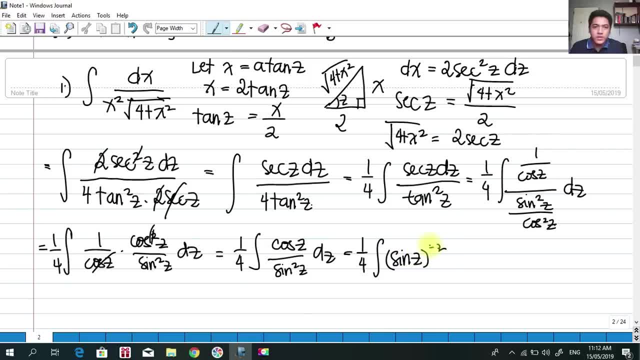 So we have 1 fourth integral of sine z raised to negative 2.. So we have 1 fourth integral of sine z raised to negative 2.. OK, Raised to negative, 2.. Multiplied by cosine of z dz. So you can see, here we can let u as sine z and du is cosine z dz. 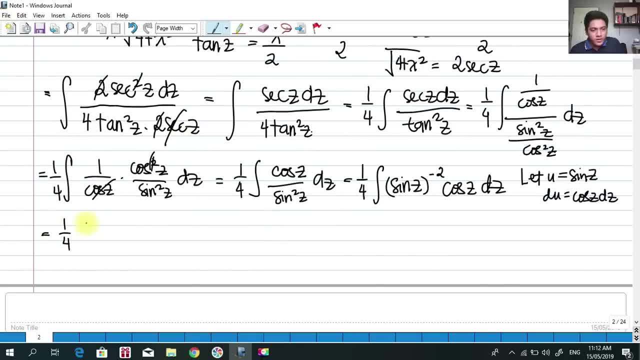 OK, So we can transform that into 1. fourth, the integral of u raised to negative 2 that du, so that we have now 1: 4 u raised to negative 1 over negative, 1 plus c, so that should be 1 over 4 u, 1 over 4 u. okay, negative 1 over 4 u, because we have a negative. 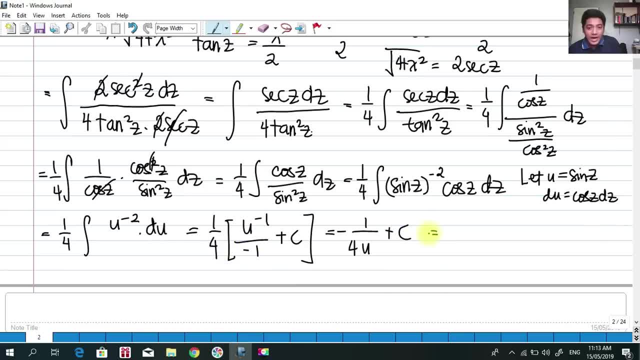 1 here plus c and substituting back u, that should be negative 1 over 4 sine of z plus c. so this is not the final answer, because this is actually expressed still in terms of z. our original integral is in terms of x. so what are we going to do is to eliminate this sine z. 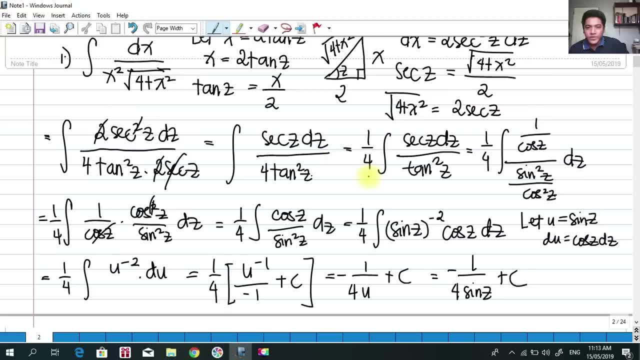 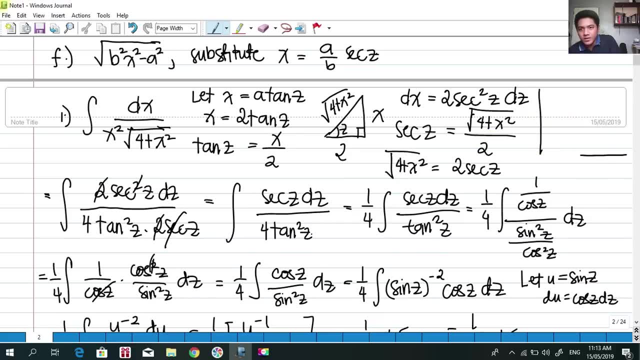 by looking at our triangle here. okay, so sine z, basically, is from our triangle here. so we're going to evaluate sine z. okay, sine z is equal to opposite over hypotenuse, right, so opposite is x. hypotenuse is square root of 4 plus x squared. 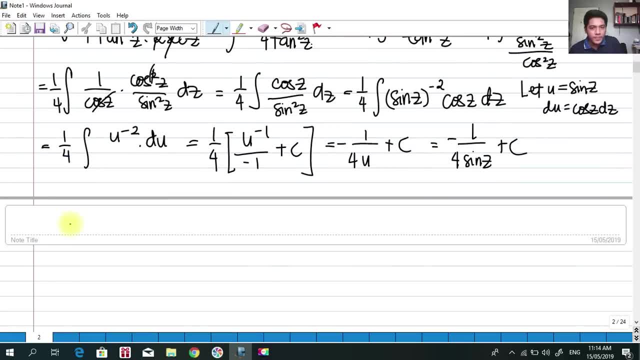 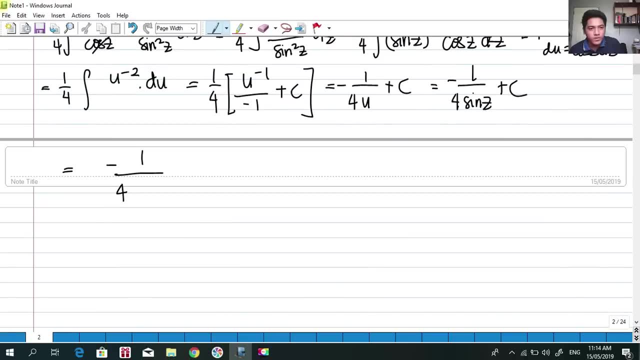 so sine z would simply be equal to what negative 1 over 4, and again that is equal to x over square of 4 plus x squared. so this is x over square root of four plus x squared, okay, plus c. and to simplify, we can get what negative of square root of four plus x squared over four x plus c. let me just rewrite: 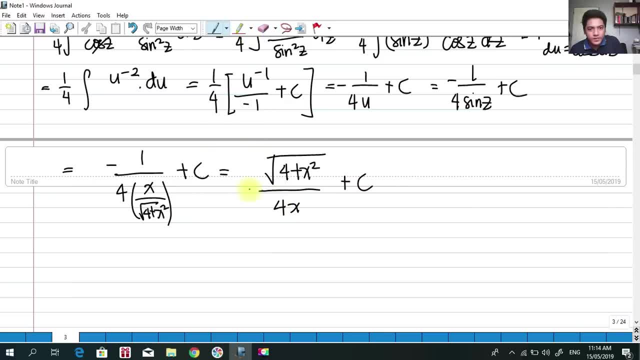 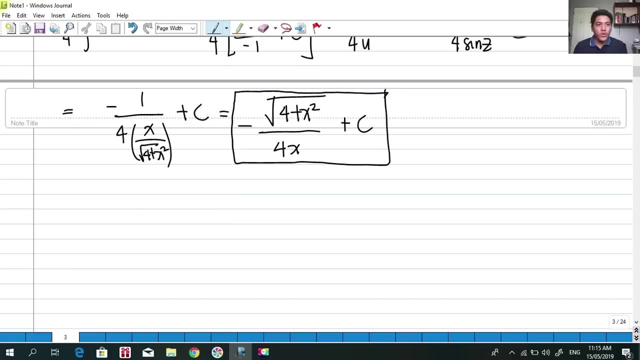 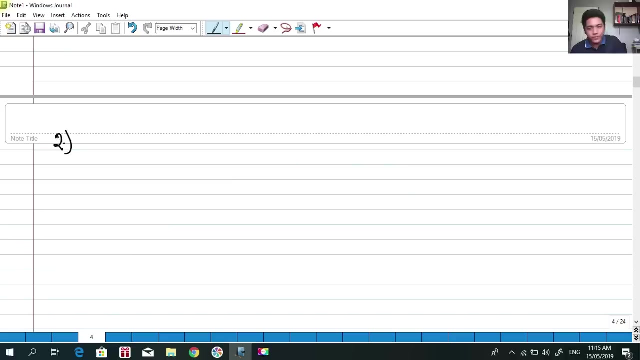 this negative more neatly here, and this is our final answer. so basically, that is problem number one. for number two problem: okay. example number two: we have now number two. that is the integral of x squared- okay, over square root of x squared minus four dx. okay, square root of x squared minus four dx. 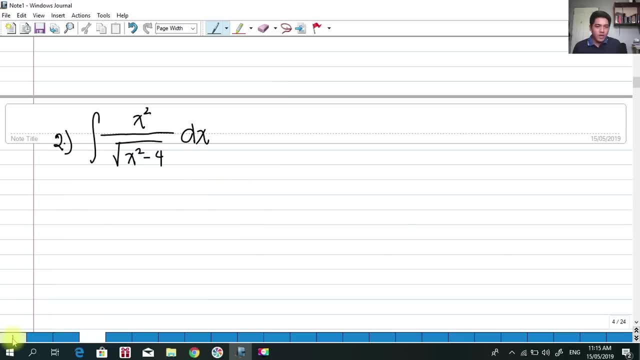 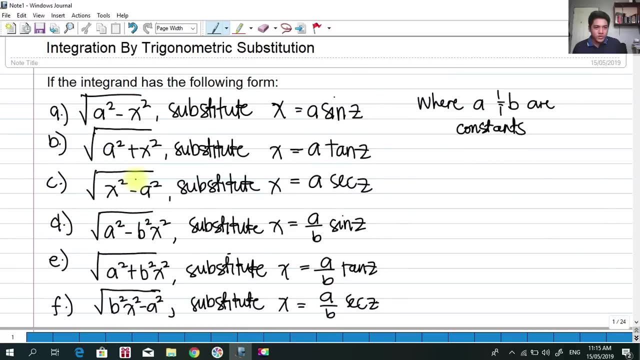 so, looking at our formula, we have the form of square root of x squared minus sum a squared. so, looking at our formula, square root of x squared minus a squared is this: because our x squared the coefficient value is one, so we can use this. we have to substitute a. 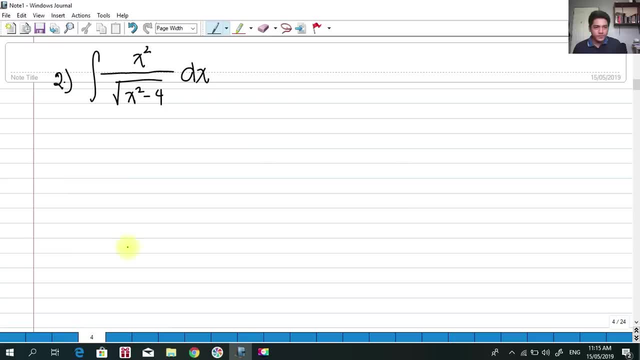 semicolon of z. x is equal to a secant of z. So we have to let: x is equal to a secant of z And x now will become a. What is our a here? The a here is 2.. Again, a squared is 4.. So secant. 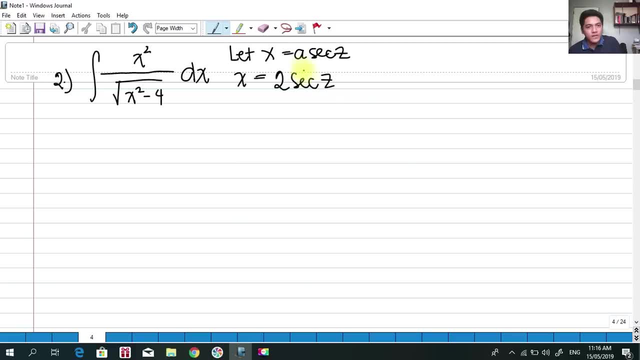 of z. And again we can derive the triangle using this equation. by isolating secant z, We have x over 2.. Secant z is equal to x over 2.. And by drawing another right triangle here we can locate: this is the z. This is the side of hypotenuse. So secant of z is: 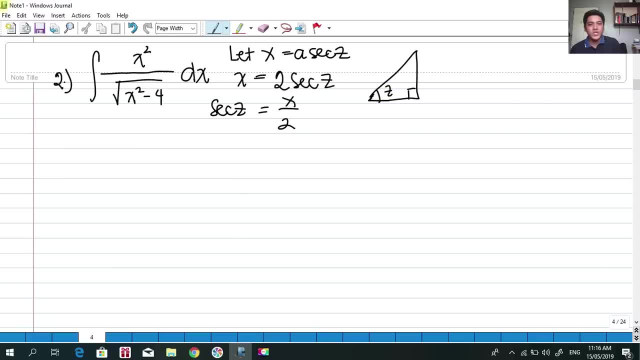 equal to x over 2.. The reciprocal of secant: 1 over secant is cosine And cosine is the pi. So if we're going to reciprocate that hypotenuse over adjacent, So secant will now be hypotenuse. 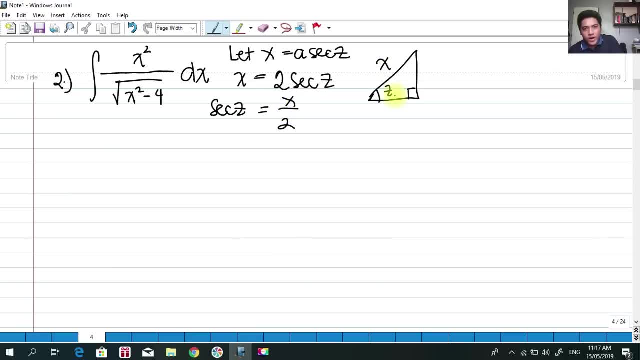 This is our hypotenuse x over adjacent side, This is 2.. And you can expect that this side actually, by Pythagorean theorem again, is x squared minus 4, which is again our part of the integral. Okay, So what do we do next? again, Yes, we're going to get the derivative. Okay, We're going. 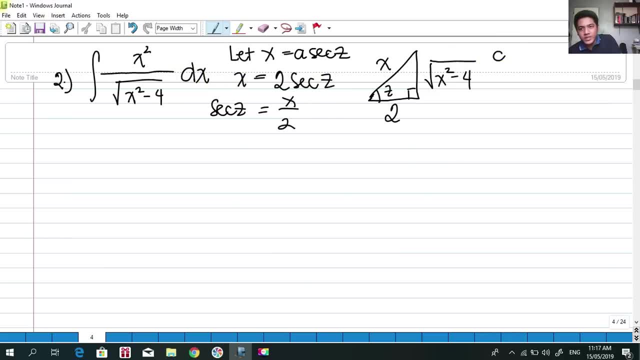 to get the derivative of this. So, in order for us to replace dx, So dx will now be derivative of 2 secant z, is 2 secant z tangent z dz. Okay, So 2 secant z of 4,. you cannot see, I think. 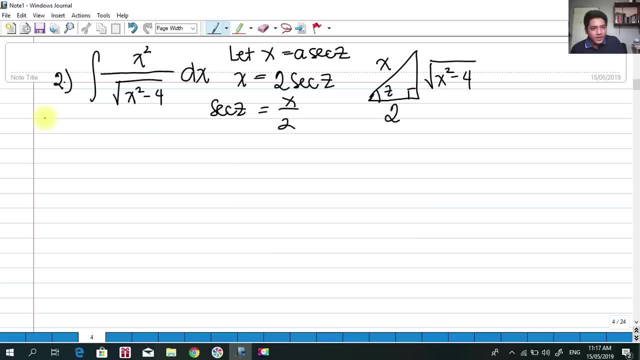 you cannot see. I will just rewrite Here: Okay, dx is actually 2, secant z, tangent z, dz. Okay, And we have now the dx. We now have the x squared. We're going to simply square this And we should get square root of x squared. 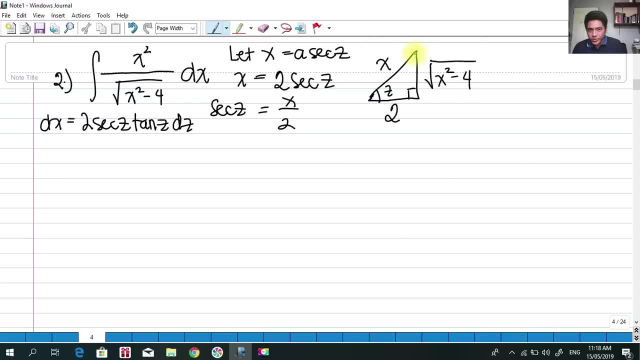 minus 4.. And again, looking at the triangle, we should avoid using the side with an x, So we have to avoid the hypotenuse. So what are we going to do? We're going to use this function, only the adjacent and the opposite. So we can use what? 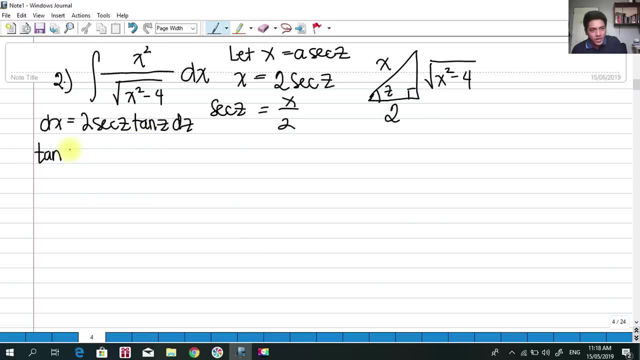 Since it has tangent here, so we can use the tangent function. Tangent of z is simply taua, opposite over adjacent. So the opposite of this z is side is x squared of x squared minus 4 and its adjacent is 2. So taua is simply square root of x squared minus 4 over. 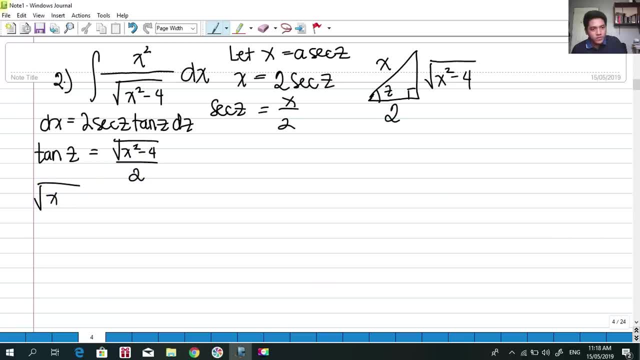 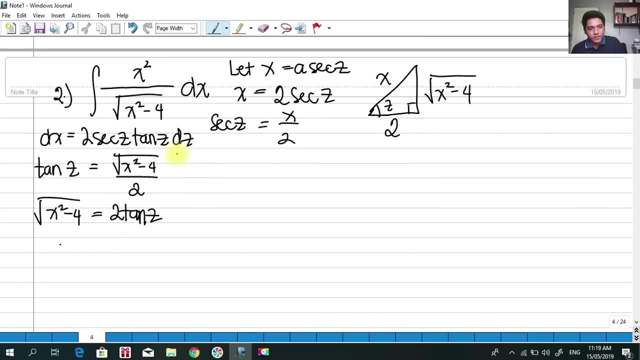 2. And we can get square root of x squared minus 4.. Square root of x squared minus 4 is 2 tangent of z, And now we can replace our integral. Okay, We're going to replace our integral. We can now have what? Let me just make a space. 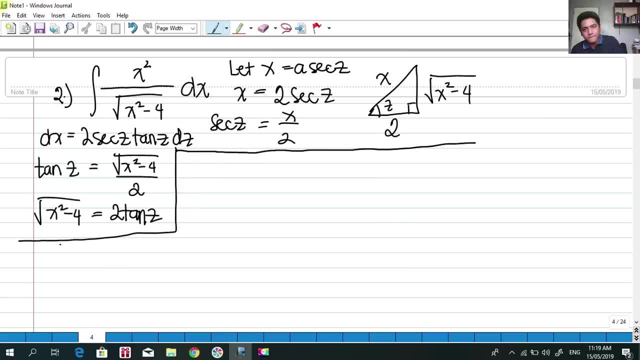 here. Okay, So we can replace the integral by simply what x squared is. we have to square the x, So we have 4 secant squared z over square root of x squared minus 4.. That is equivalent to 2 tangent of z, Okay, Multiplied by dx, And our dx is simply this: 2 secant z tangent. 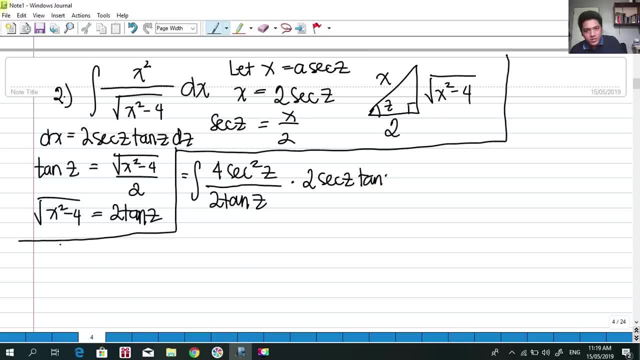 z 2 secant z tangent z, dz. As you can see here, 2 tangent z will cancel, And we can cancel by this. Okay, And you are left with the numerator. What Integral of what? 4 secant. 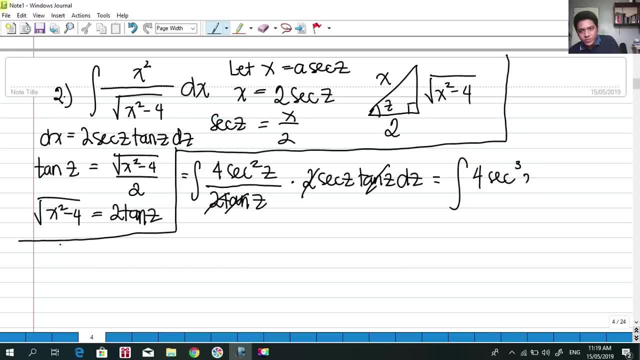 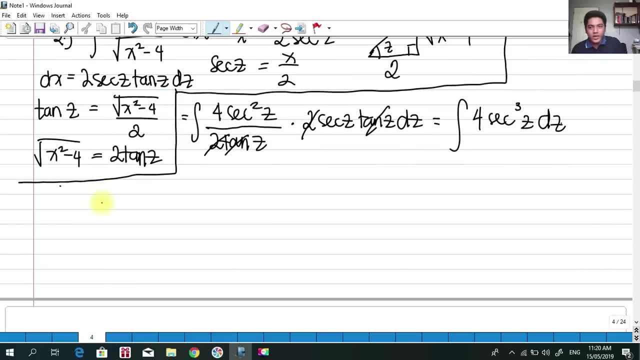 squared z times, secant z. secant cube z dz. Okay, So that is now our integral. So we can integrate this using integration by parts. So we have now integral of, let's say that is 4. 4. integral of z. 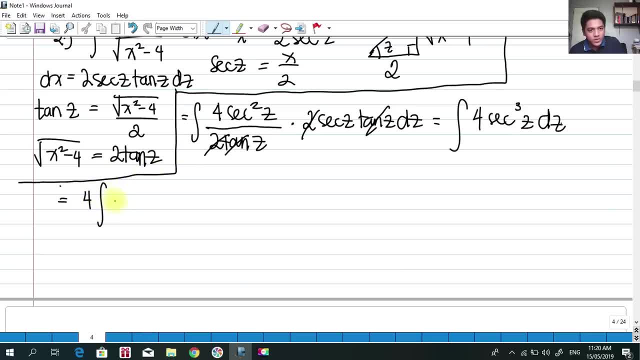 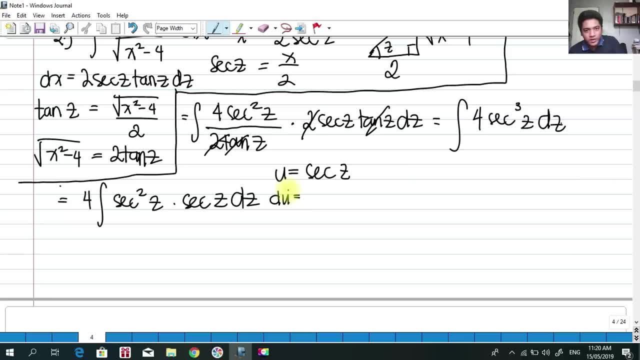 it's the same. So getting du here, and the derivative of this is secant z, tangent z, Okay, And of course dz, And of course our dv would now be the remaining Okay, Which is actually secant squared dz. So in u we use only secant z, because this is already readily. 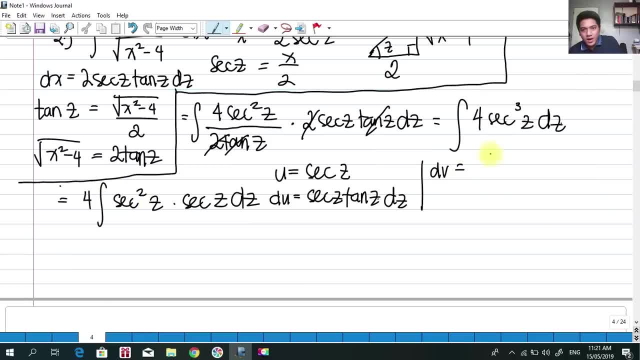 integrable. Okay, So dv is secant squared z, dz, And if we integrate that both sides, we have v now is equal to the integral of this is basically 2.. Okay, So secant squared z multiplied by secant z, tangent z And applying the formula uv minus. 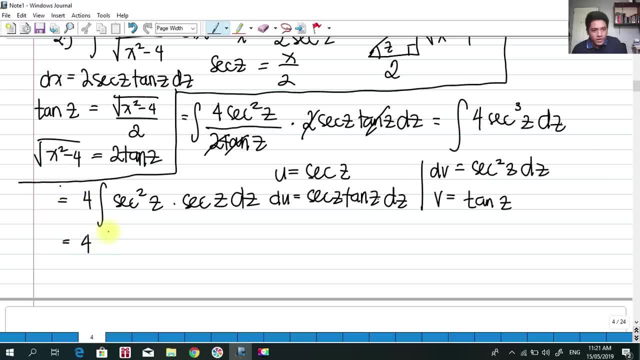 vdu. we have now what 4 multiplied by again, let me just rewrite the formula: uv minus the integral of vdu. That is our formula for integration by parts. We have 4 times the u times v. u is secant z times v Secant z tangent z Agreed. Secant z tangent z minus. 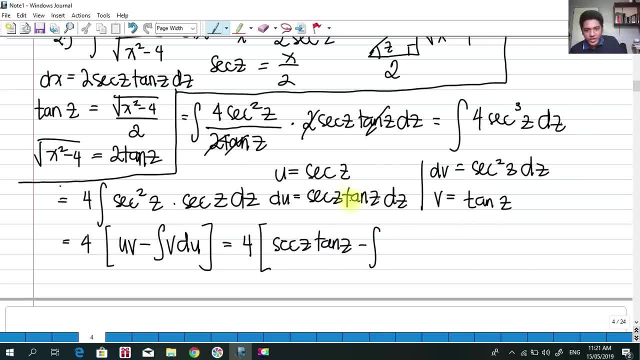 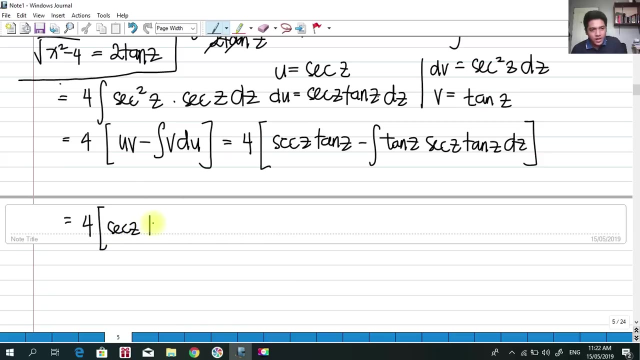 the integral of the v, which is tangent z, Tangent z, Then du, which is secant z, Secant z, times tangent z, dz. Okay, Uv minus vdu. integral of vdu. Okay, So what will happen here is that we have 4 secant of z, tangent of z minus. we can combine the total sine: of z, That's just v. So we now have 2 secant z times z. So this is our 2 secant z times vdu. Okay, We now have 4 secant of z, tangent of z minus, we can combine the total sine. 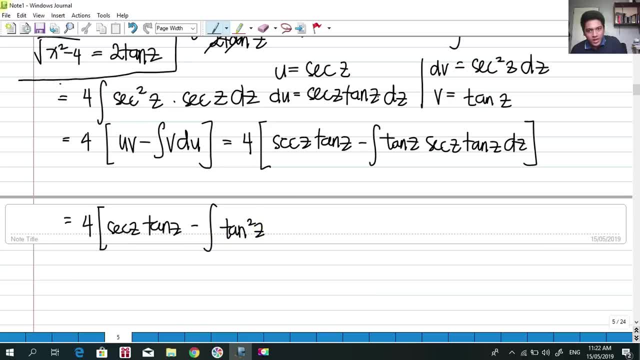 tangent squared. okay, tangent squared z times secant z dz, and from here we can use the. we can actually convert this into tangent squared z. remember: tangent squared z is equal to secant squared z minus one by this identity. so we have. now we have to distribute four. 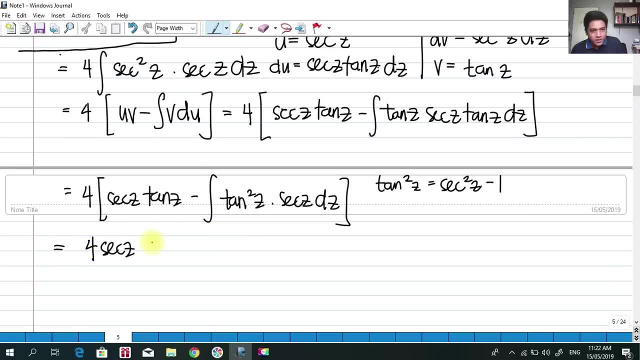 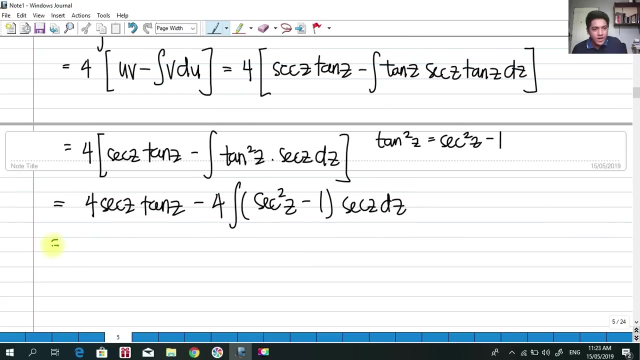 can we distribute, yes, four secant z, tangent of z minus four, integral of what secant squared z minus one, because that is equivalent to tangent squared z multiplied by secant z dz. okay, so, i'm sorry. okay. so again, by techniques, we have four secant z tangent of z. and basically, what if we, if we uh distribute? 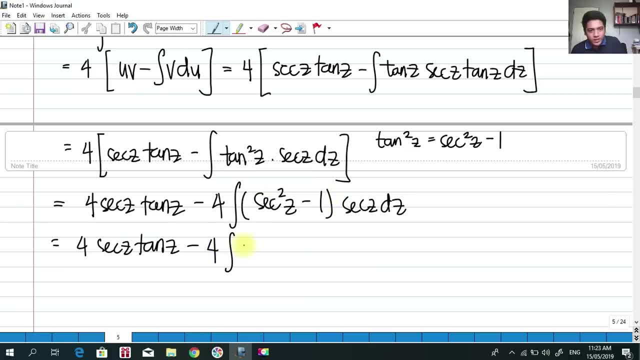 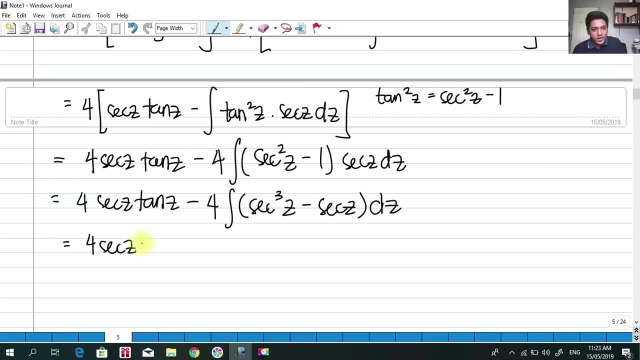 the secant z to this we will be having, minus four, the integral of secant cubed z minus secant z, and that is integrated by dz. as you can see, here we can distribute the integral. so we have four: secant of z, tangent of z. 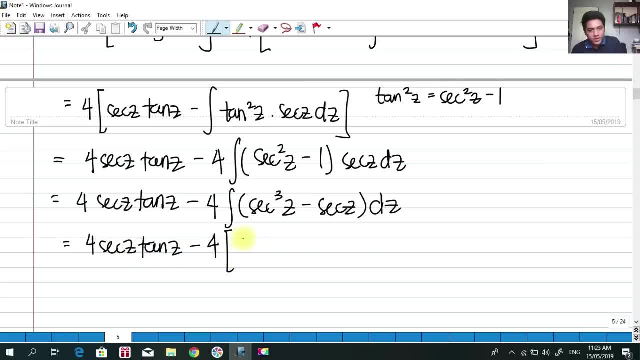 z minus four, of course, the integral of secant cubed z dz. okay, let me just uh distribute again the negative four. so this would become what? of course this would become negative four. integral of secant cubed z dz. so if, because of this one, the fourth integral gives minus four, 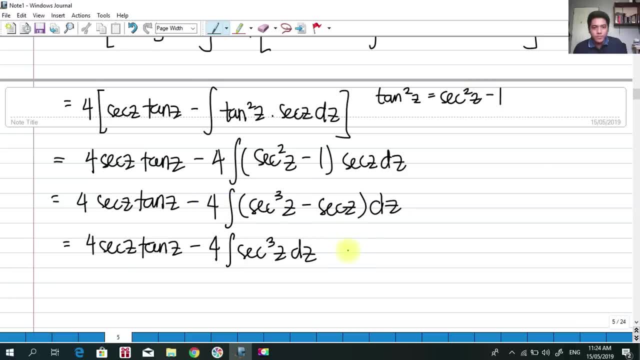 okay minus four. okay, minus negative. four times negative will become positive. four secant of z dz. okay, we have distributed the four here. okay, so this become positive, because relacion four times하비에 대해 영상과 연결된 잂�을. 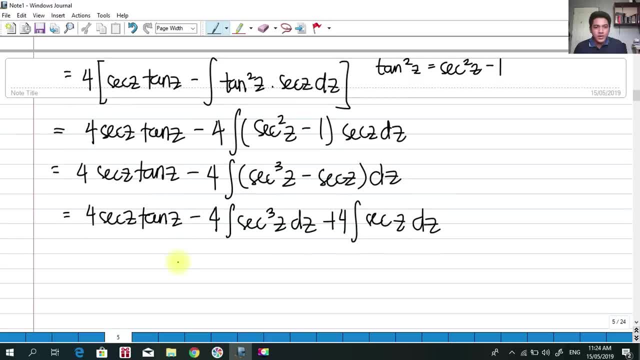 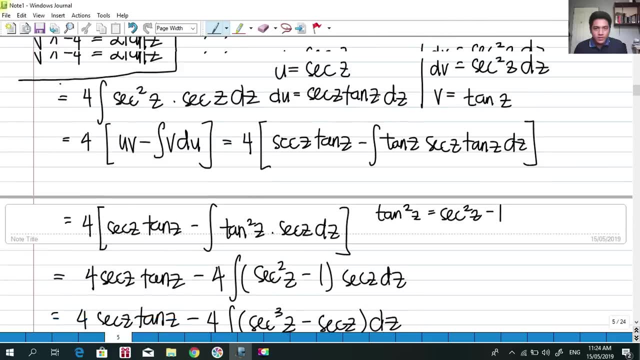 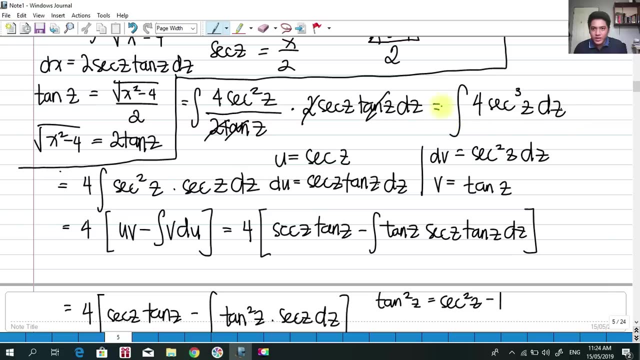 negative four times, this negative will be positive. okay, so, as you can see here, Our integral yields to this again secant cube of j dz, wherein, of course, we started with that again. Of course, this is our original integral, okay. 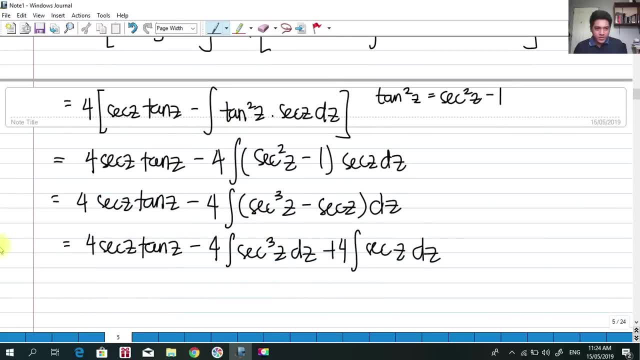 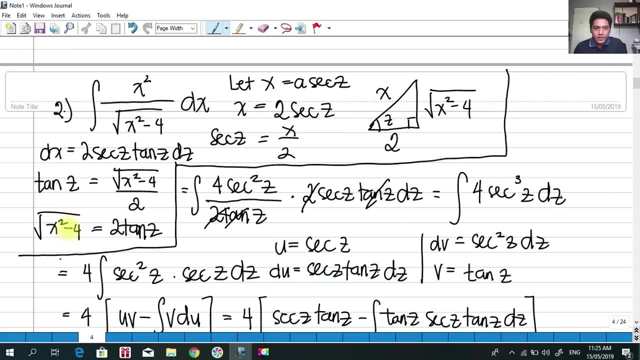 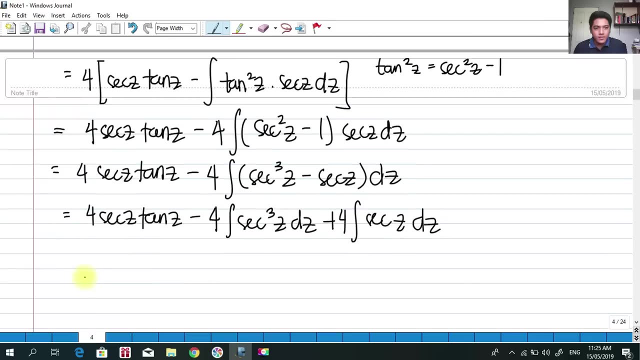 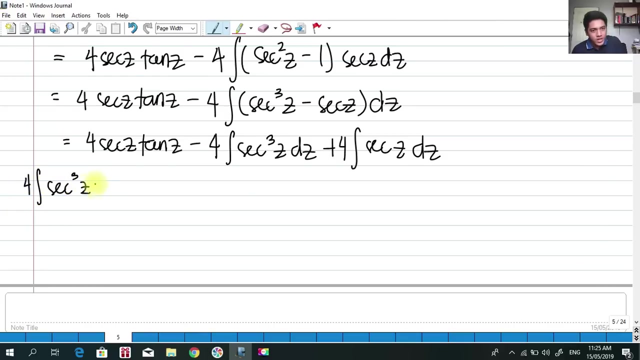 And we return back to this. So basically, okay, let's copy this side. okay, Let's copy: to end this integral, To end this integral. okay, We're going to copy that. So that is equal to 4 integral of secant cube j, dz and it is equal to this integral. agree, 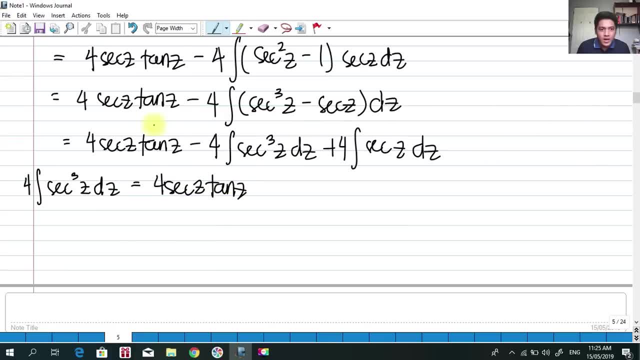 Because this integral came up when we used IBT on this integral. So this must be equal, okay, Minus 4 integral of secant cube j dz. plus 4 integral of secant j dz. What are we going to do to eliminate this? 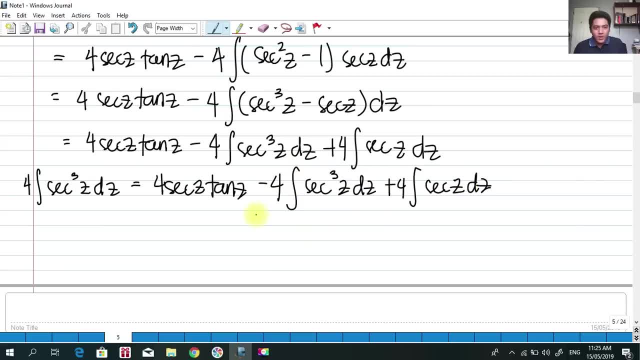 Because this will yield to an unlimited IBT. we're going to add plus 4 integral of secant cube j dz on both sides of our equation: Plus 4 integral of secant cube j dz. Okay, what you add on the left is what you add on the right side. 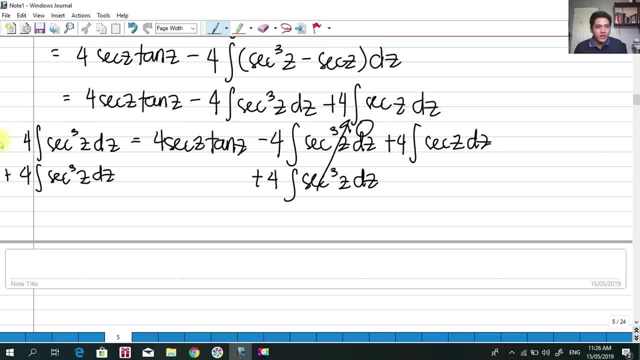 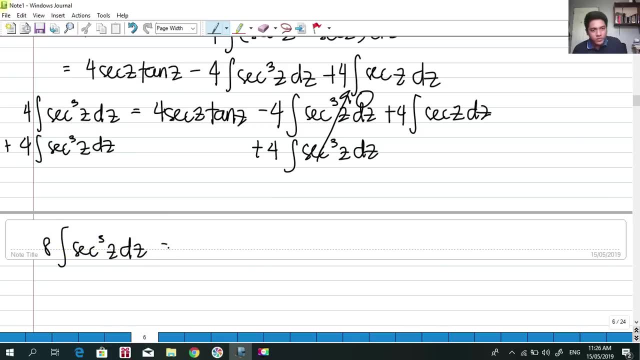 So this would now become 0,. okay, And here, if you're going to add this, We have now 8 integral of secant cube j dz, and that is equivalent to 4 secant of z- tangent z plus 4 integral of secant of z dz. okay. 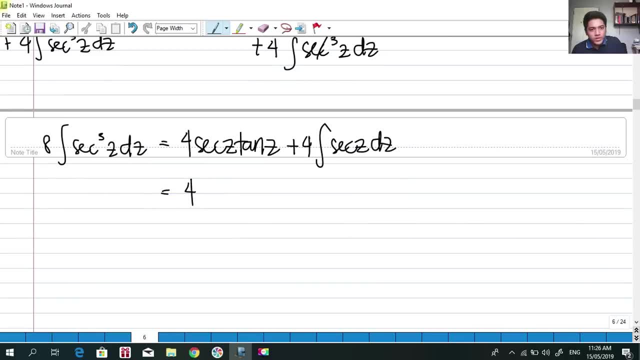 And what are we going to do? 4 secant of z, tangent of z. Can we integrate this secant? Okay, What is the integral of the secant? Oops, The integral of secant is actually what? 4 ln of secant of z plus tangent of z plus c. 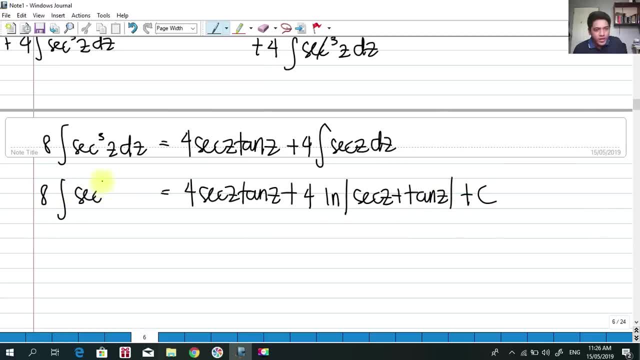 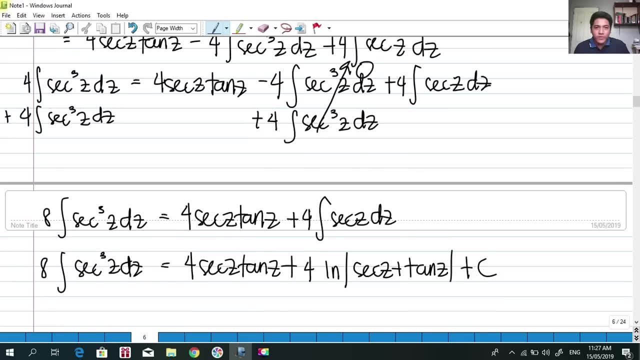 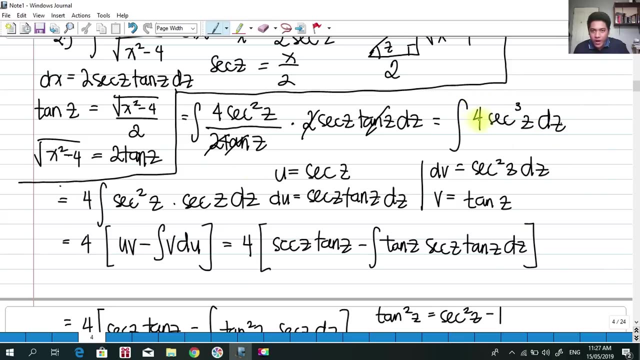 And, as you can see here, the right side is equivalent to 8 secant z, dz. But what we are after is actually not this. We are after for the integral of what, The integral of 4 secant cube z, Or this factor of 4 outside the integral. 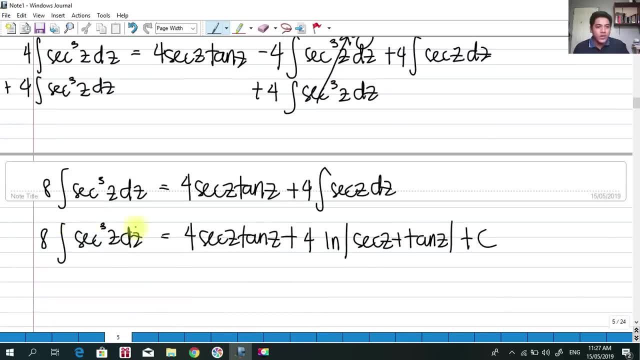 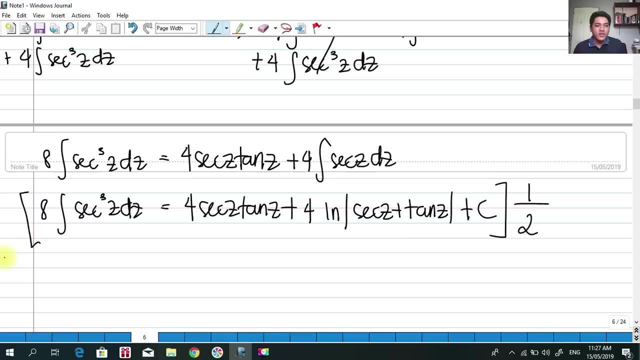 We are after that. So we have to make this left equation equal to 4 secant cube z. So what are we going to do? By simply dividing both sides? by what? By 2, actually. So if we divide that, this would now become our original integral a while ago: 4 secant cube z dz. 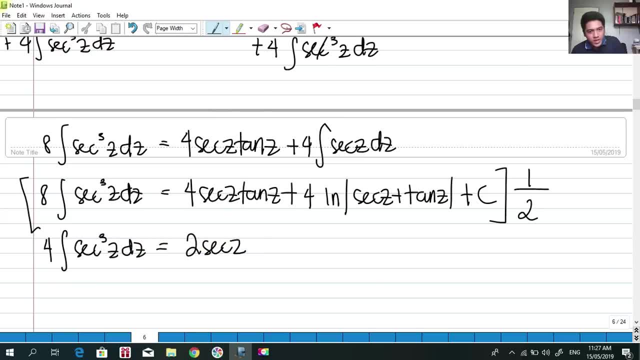 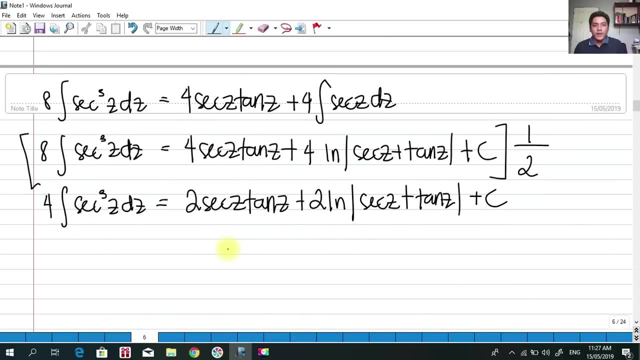 So 4 over 2 is 2 secant z, tangent z plus 4 over 2, that is 2 ln of secant z plus tangent z plus c. Now this is not our final answer, because we have to. what? 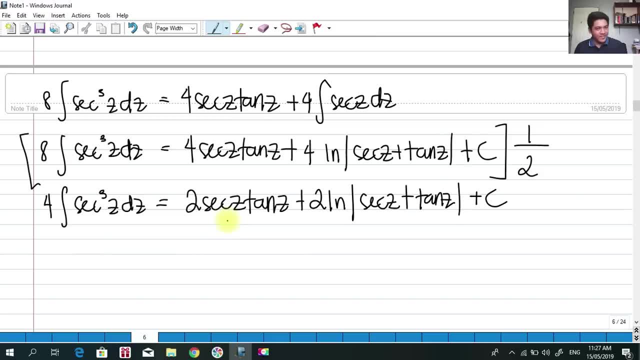 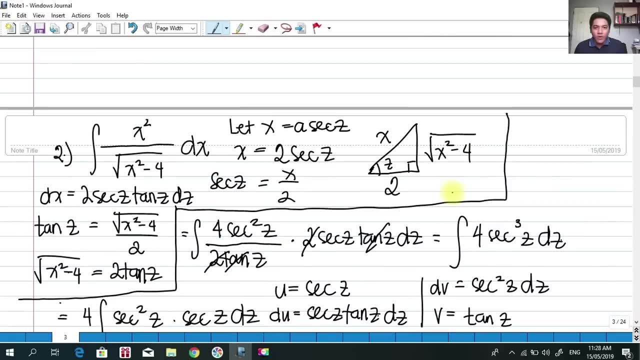 To translate this z into x again And again. what are we going to do? We need secant z and tangent z. at least What we are going to do, We are going to get back on this triangle. Okay, So again, we already got the secant z. 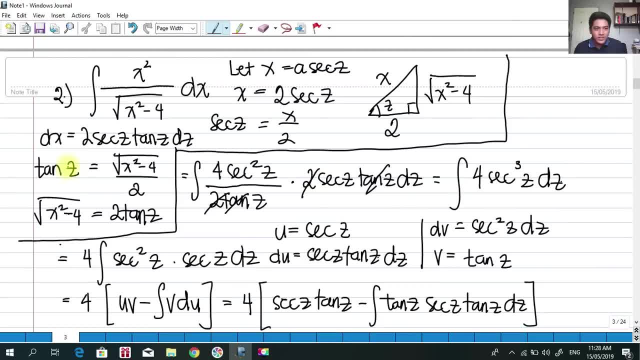 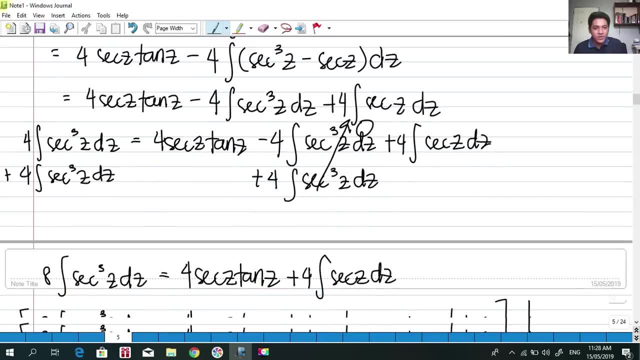 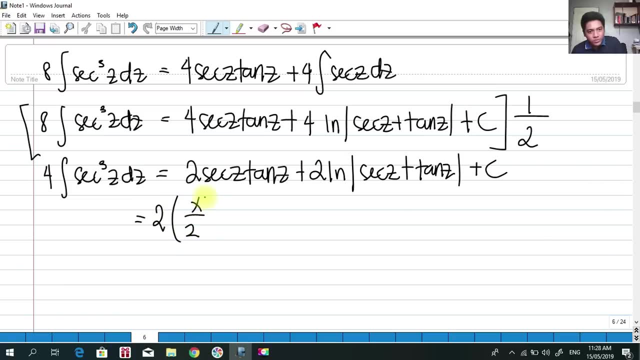 And secant z is equal to x over 2.. And tangent z is square root of x, squared minus 4 over 2 here. Okay, So secant z is x over 2.. So we have here 2 times the x over 2.. 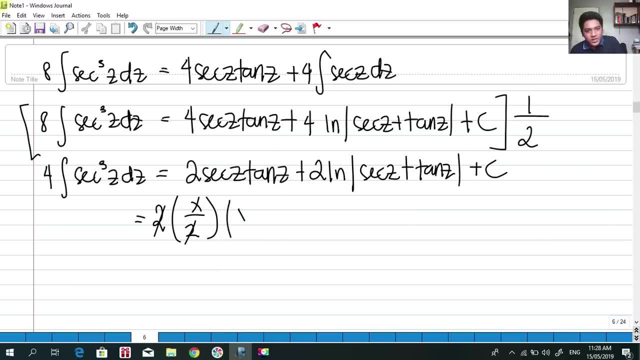 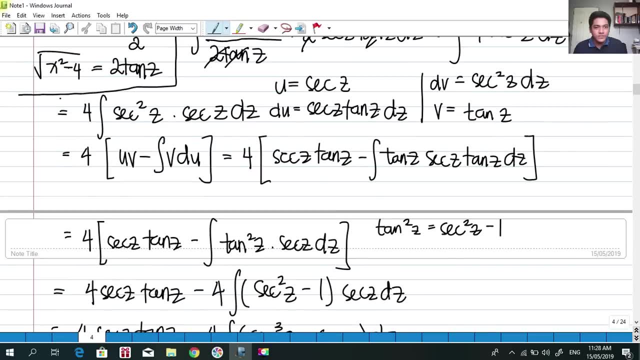 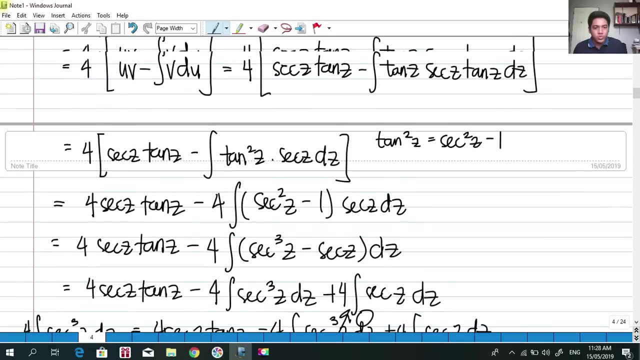 Those 2 will cancel Times the tangent z. Tangent z is equal to x squared minus 4.. Okay, I'm not mistaken. Is that minus 4?? Okay, x squared minus 4 over 2.. Okay, Over 2.. 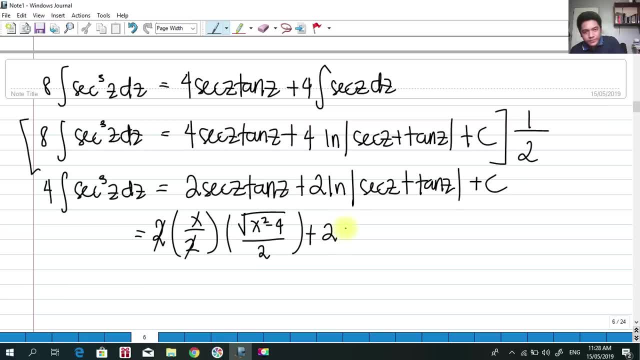 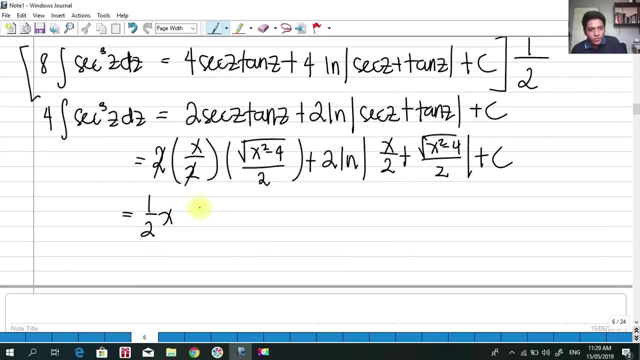 Over 2 plus 2 ln of the absolute value of secant z is x over 2 plus square root of x squared minus 4 over 2 plus c, And, simplifying, we have now 1 half, 1 half, 1 half of x multiplied by x squared minus 4 plus 2 ln. 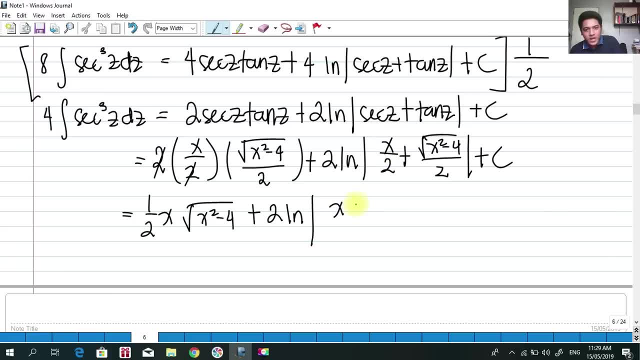 The absolute value. since they have the same denominator, We can simply add them: x plus x, squared Square root of x, squared minus 4 over 2 plus c, And this should be our final answer. Okay, Okay, Okay, For our third example. 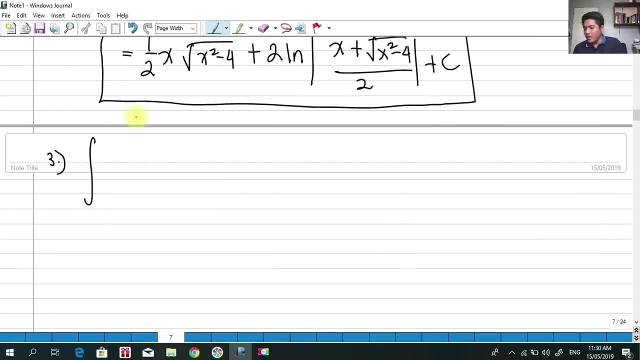 For our third example, We have to get the integral of the square root of 9 minus 4x squared over x- Oops, Over x, Multiplied by dx. Okay, And again, you're going to look back. We're going to look back on our formula. 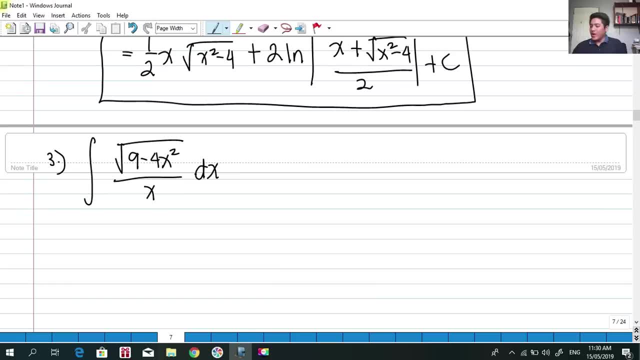 Well, I'm going to copy it. You must copy it. So what will happen, class, is that this integral has a form of what, A form of a squared minus b squared, x squared, And this is basically equal to what. 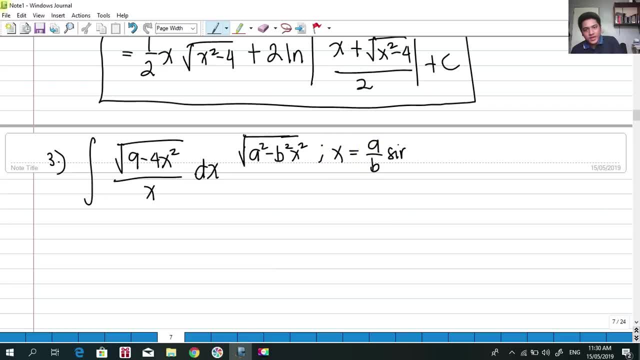 x is equal to a over b sine z. Okay, So we're going to use this equation, So our x will be simply what Our a here in this case is not 9 but 3 over, not 4 but 2.. 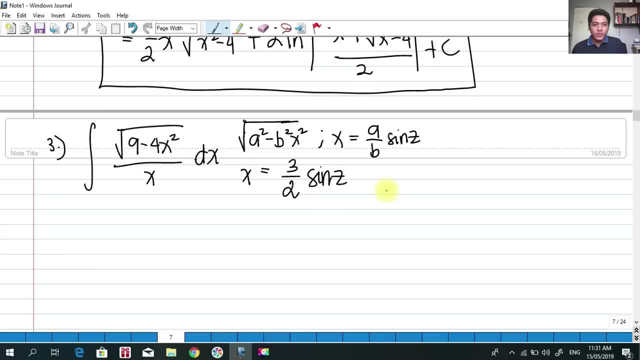 3. So we have sine z And well, of course, again, we're going to derive our triangle from this equation, So that if we're going to get the sine of z, that is equal to 2x over 3.. 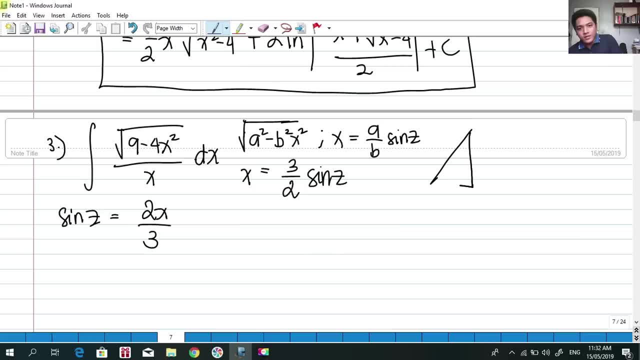 And if we're going to draw the triangle right triangle of that. So now we have, this is the hypotenuse side, This is sine z, So this will be our angle, z here, So z is so Opposite is 2x. 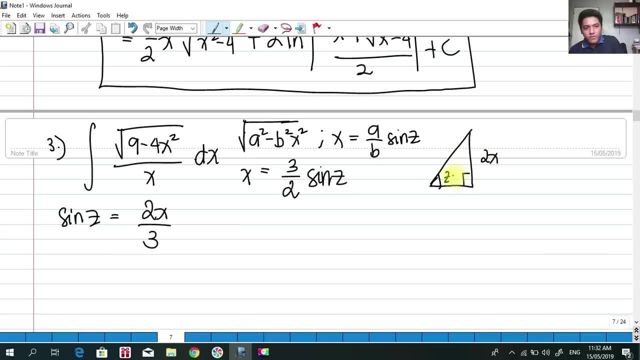 Opposite side of z is 2x. This is the opposite side over hypotenuse is 3.. So that this side, this adjacent side, is now- I'm pretty much sure that that is square root of 9 minus 4x- squared. 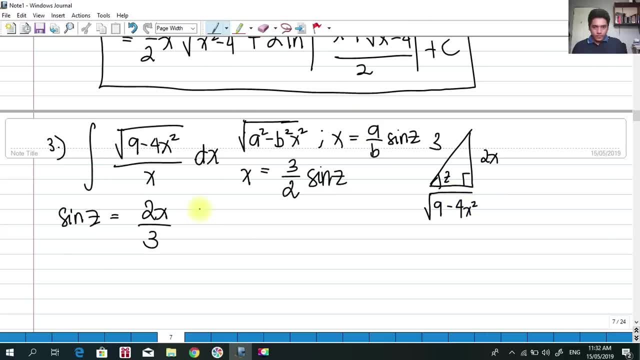 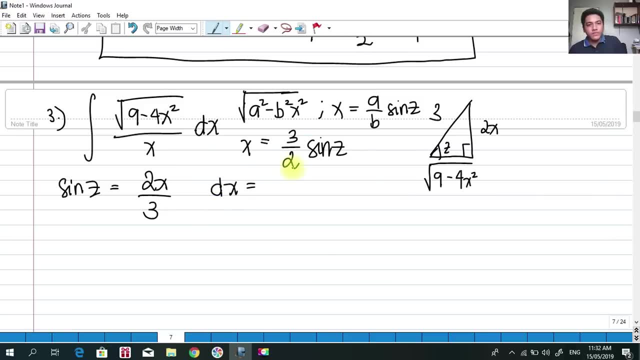 Okay, So, and again we're going to get the dx. dx is derivative of 3 halves sine, z is 3 halves Cosine of z. And again we're going to get square root of 9 minus 4x squared. 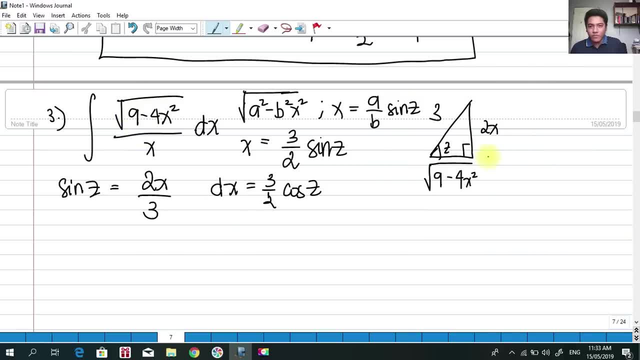 So, as you can see here, as much as possible in this triangle we have to avoid the term that has an x, which is this side Opposite to angle z. Okay, So we're going to use either this and this side. 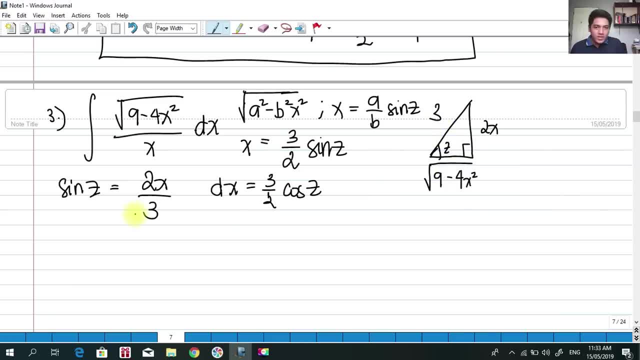 So adjacent and hypotenuse. So based on our x and dx, we can use the cosine function. So for us to be Cosine, z is adjacent over hypotenuse. So the adjacent side of z is 9 minus 4x squared over the hypotenuse is 3.. 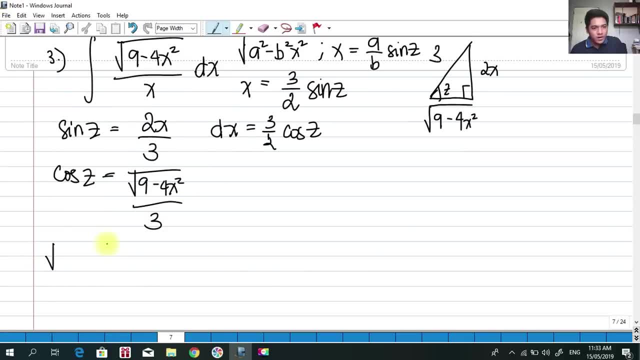 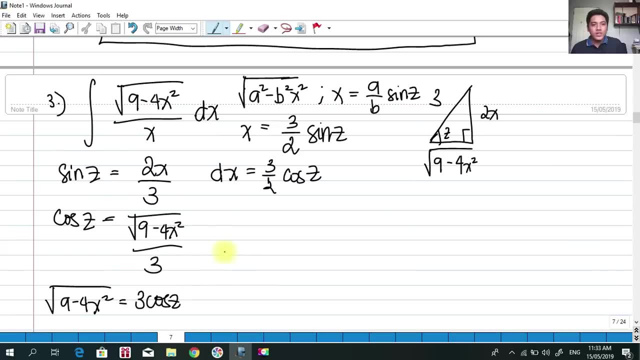 So that if we're going to get square root of 9 minus 4x squared, that is simply equal to 3 cosine of z, And now we can substitute it to our integral. Okay, So our integral will now be: 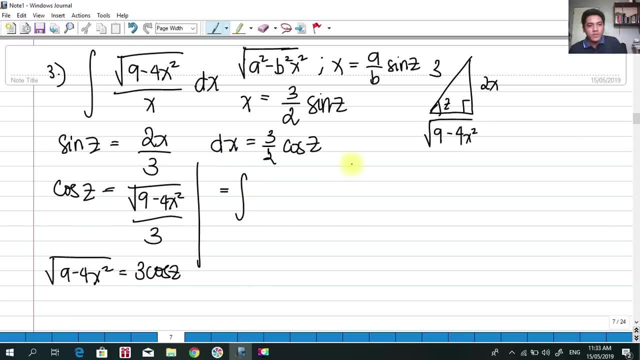 Okay, Okay, Our integral will now be: square root of 9 minus 4x. squared is 3 cosine of z, over what? The x value, that is 3 halves sine of z, And the dz or dx, is equal to 3 halves cosine of z. 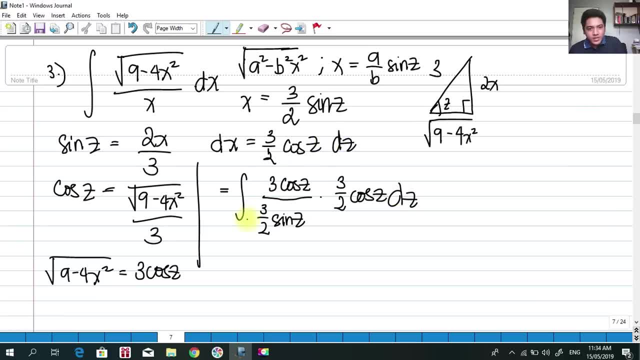 dz. This has a dz. Okay. So what happens is 3 halves will cancel. Okay, So that we have now the integral of 3.. Cosine squared z Cosine times. cosine. Cosine squared z over sine z dz. 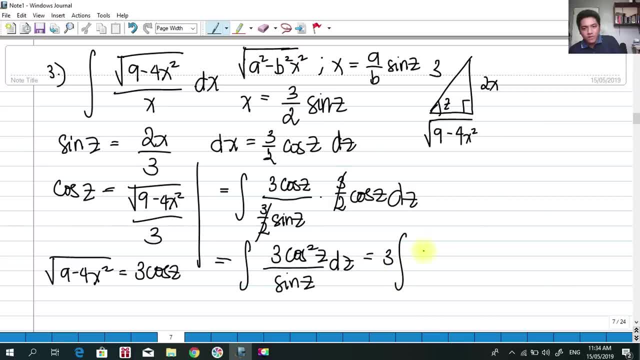 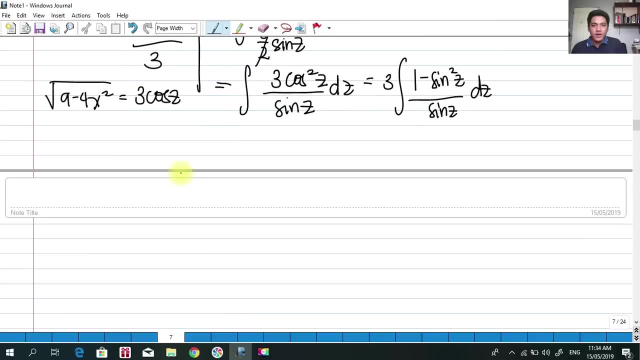 We can factor out 3 outside of the integral. 3 integral of cosine squared z is equal to 1 minus sine squared z over sine z dz And we can factor out basically the integral here. We can separate, So we have 3.. 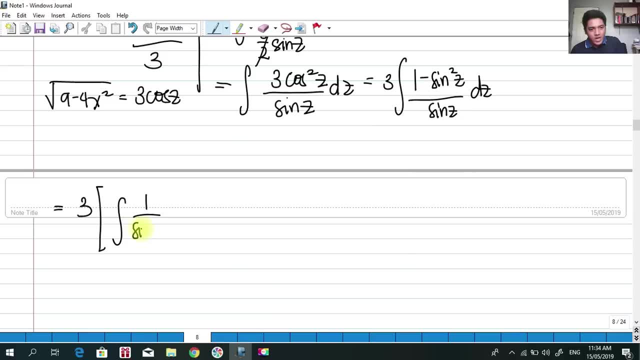 Multiplied by the integral of 1 over sine of z dz, minus the integral of sine squared, z over sine of z dz. So, as you can see, sine squared will be cancelled by this sine on the denominator. So we have now 3 integral of 1 over sine. 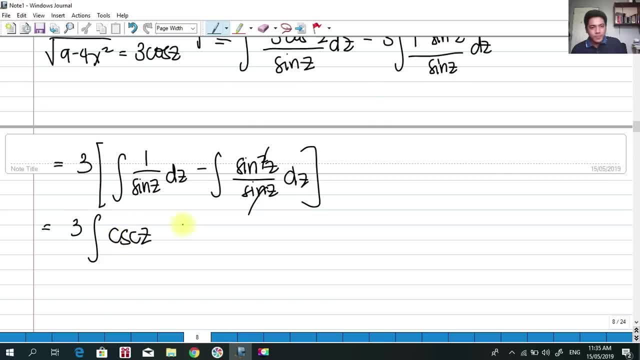 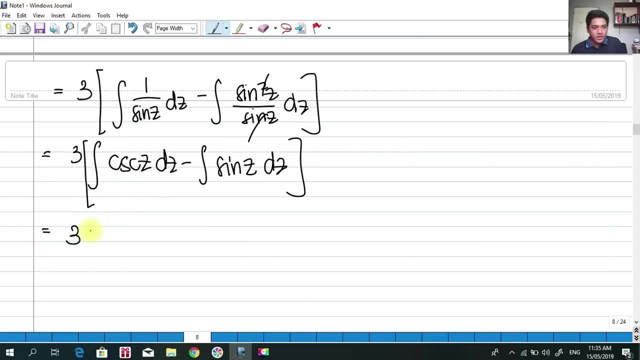 1 over sine is equal to cosine z dz. Okay, Again, Minus the integral of sine z dz. To integrate that: So integral of cosine is ln. Absolute value of cosine z minus cotangent z Minus Okay. 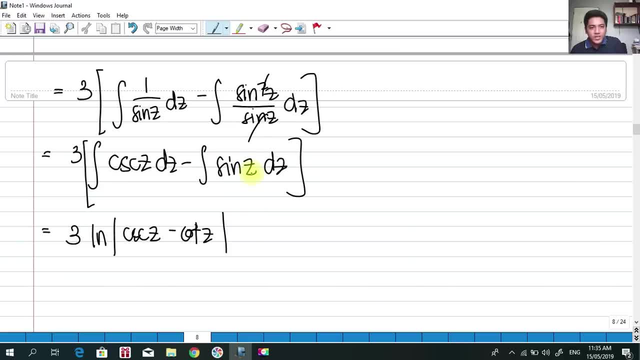 The integral of sine z is negative cosine z, So negative cosine z times the negative will become positive. Okay, And we are going to distribute 3 here, So that would be plus 3 cosine of z plus c. Of course, this is not our final answer. 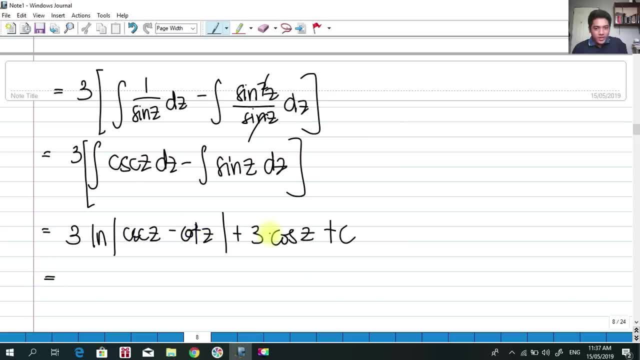 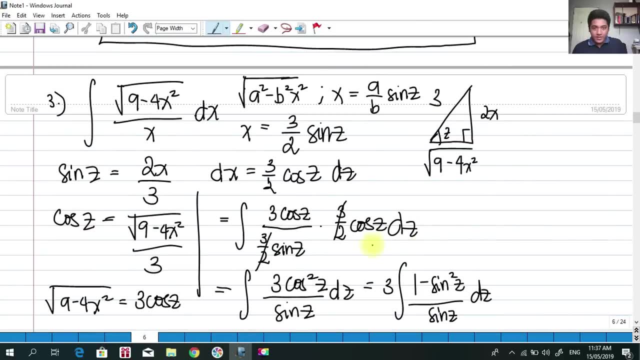 So we need to get cosine z and cotangent z and cosine z. Well, of course, in our what, In our triangle. So we have now already the cosine z, So we should get cosine, So we should get cosine. 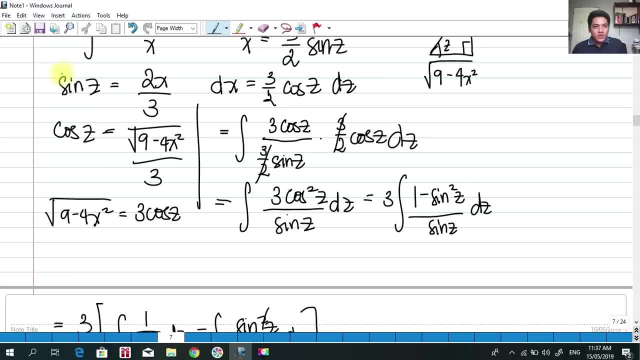 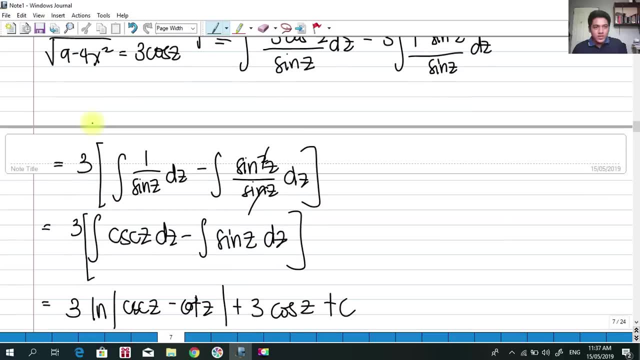 And cotangent. So we have here sine of z. So to get cosine of z, simply we need to get the reciprocal of this. Okay, So the reciprocal of this is 3 over 2x, So 3 ln. 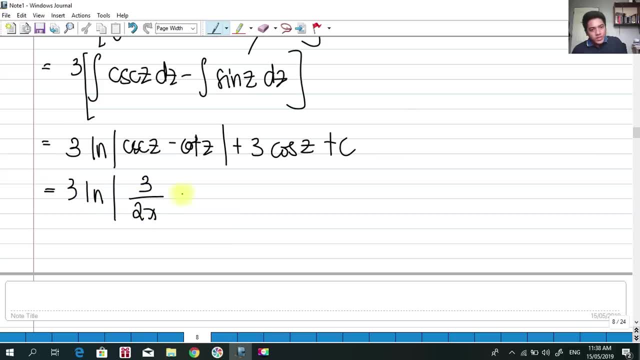 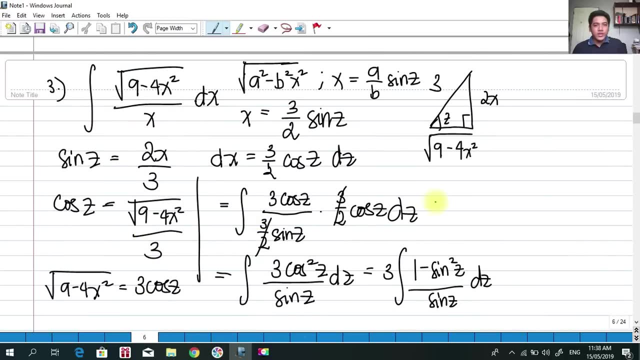 Cosine z is simply equal to 3 over 2x minus cotangent z. Cotangent z is basically: if tangent is tau Opposite Over adjacent, Cotangent is adjacent over opposite, So that should be the cotangent of z. 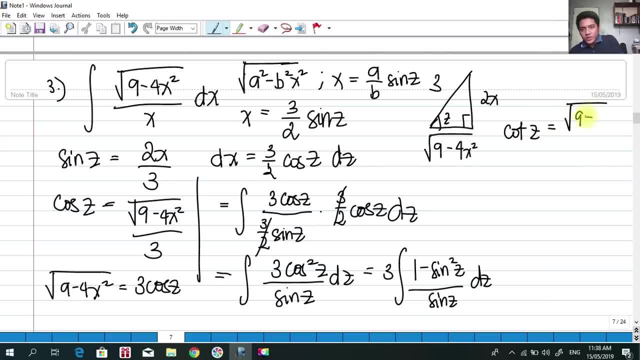 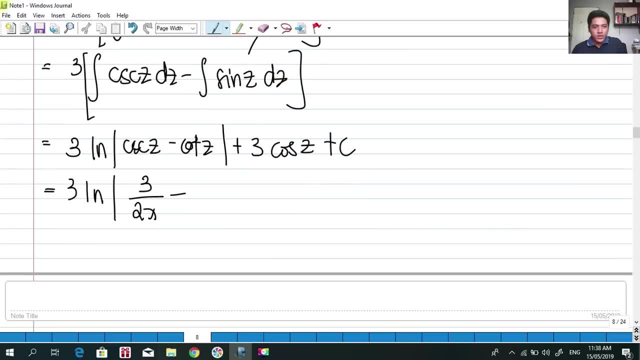 Okay, Simply adjacent: Square root of 9 minus 4x squared over opposite, Over 2x. So we can substitute it here. So cotangent z is square root of 9 minus 4x squared over 2x plus 3, cosine z: 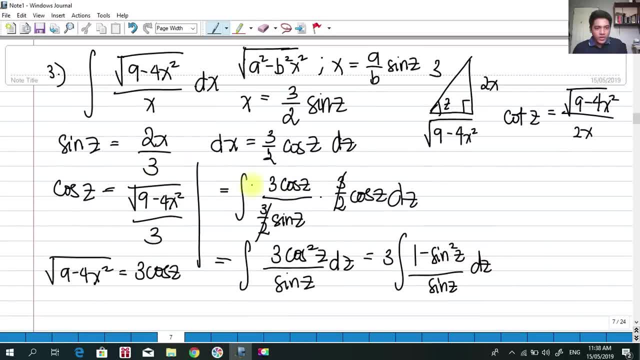 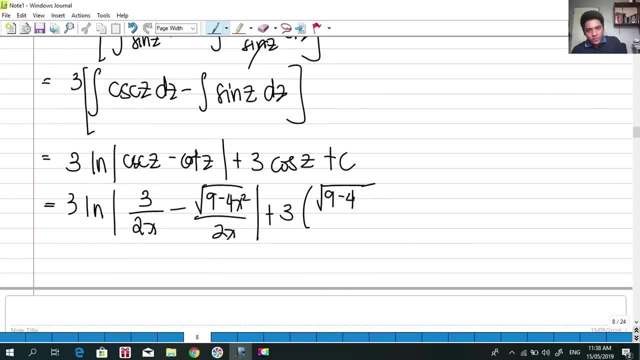 Cosine z from our figure here or from this, is equivalent to square root of 9 minus 4x squared over 3.. So we have square root of 9 minus 4x squared over 3 plus c. Simplifying 3s will cancel. 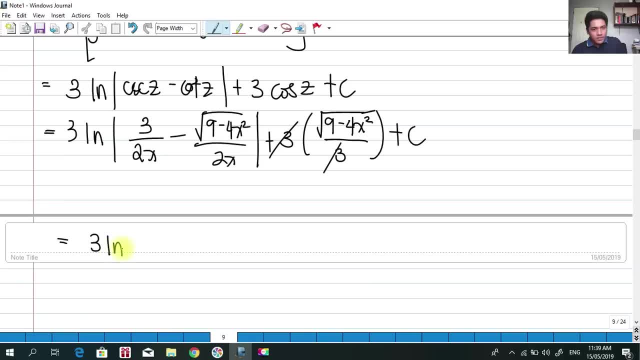 Okay, So we have now the final answer as 3 ln absolute value of 3 minus square root of 9 minus 4x squared over 2x plus the square root of 9 minus 4x squared plus c, And that should be our final answer. 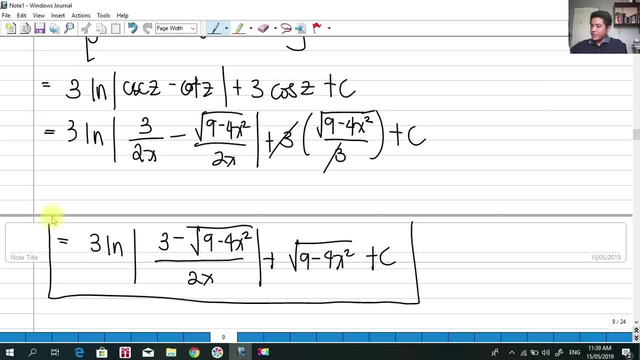 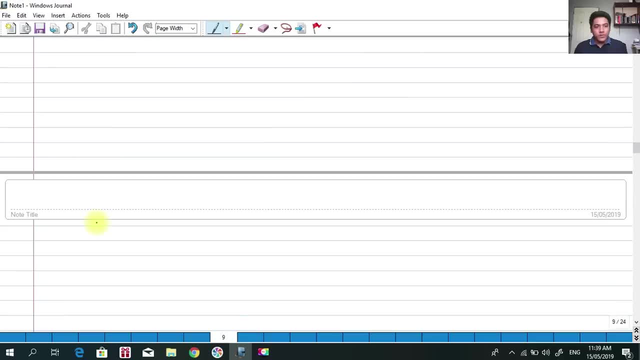 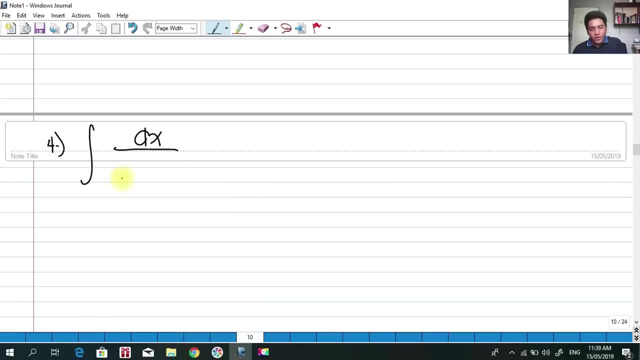 Okay, So for number 4.. By the way, this video has 5 problems, So that you will be really practiced. Okay For number 4, what are we going to do is find the integral of dx Over x times the square root of 9 plus 4x squared. 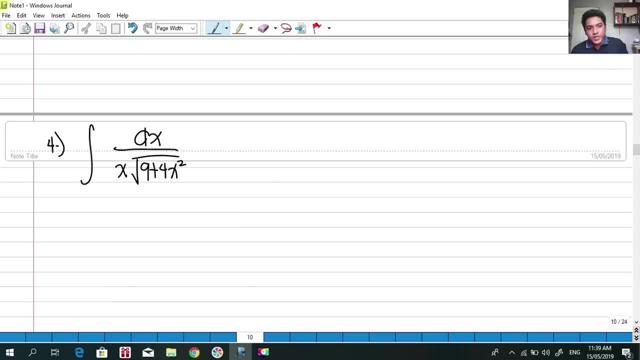 Okay, And if you're going to look at our formula, this is a form of square root of a squared. Okay. Square root of a squared plus b squared. Okay, Because we have here a coefficient of x that is not equal to 1.. 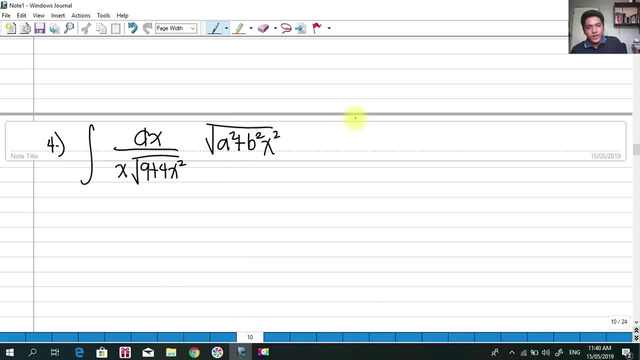 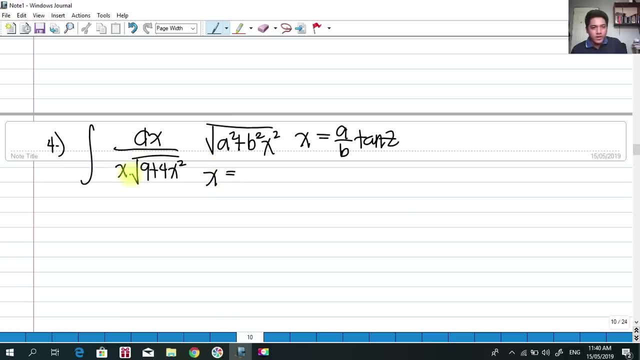 So if we're going to let, x is equal to a over b, our a here is not 9, but 3.. Our b here is 2 tangent of z, And again from this equation we're going to derive the triangle. 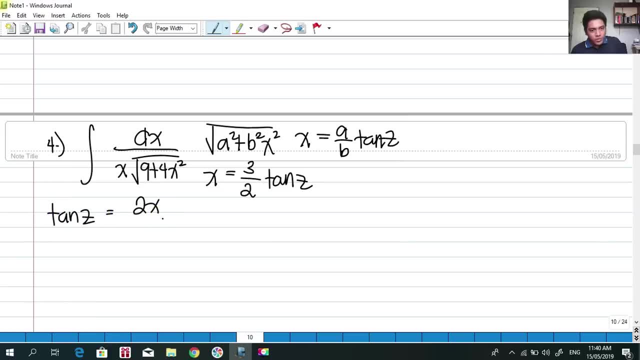 So tangent of z is equal to 2x cross multiplication over 3.. So if we're going to draw our triangle, So if we're going to draw our triangle here, okay, so this is our z. So tangent is tau. opposite side is 2x over adjacent is 3.. 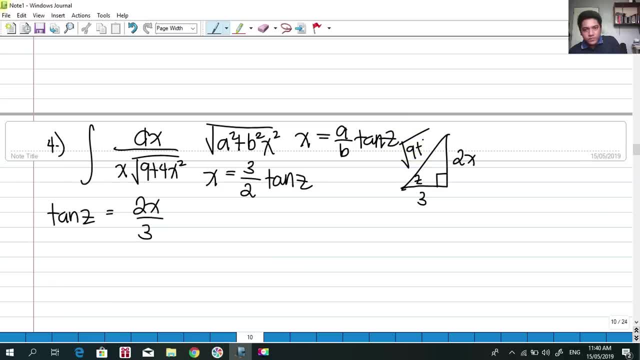 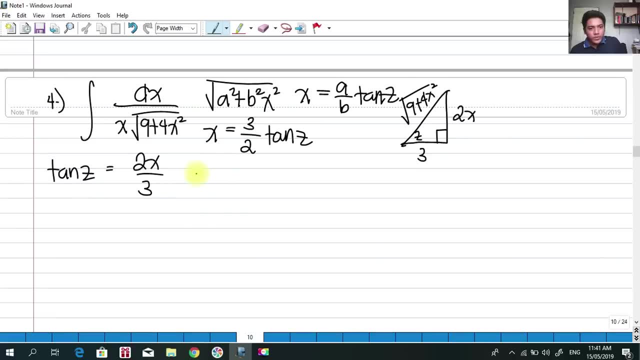 So, therefore, this side is 9 plus 4x squared. Okay, So, and again, after that we're going to derivative, or get a derivative of this: x with respect to x on the left side and with respect to z on the other side. 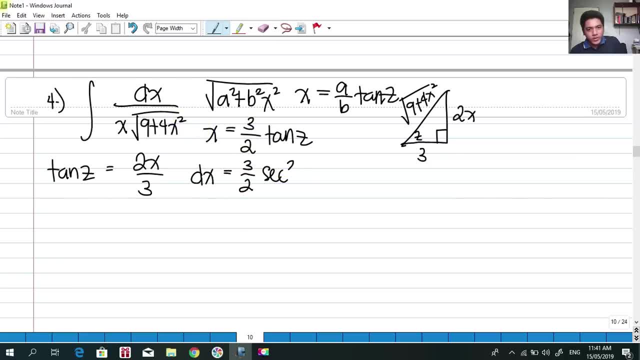 3 halves, 3 halves The derivative of tangent z. The derivative of tangent z is secant, squared z, d, z And, of course, what we are after, we get the x, we get the dx and we have to get the. 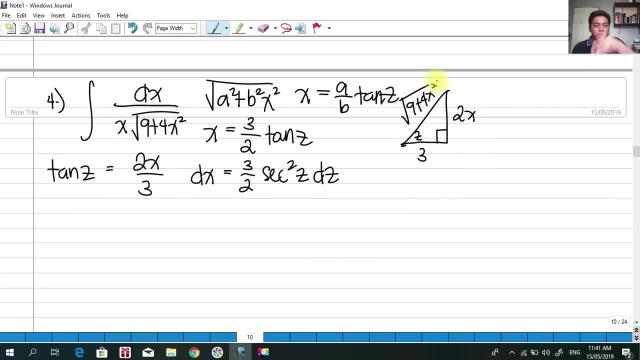 square root of 9 plus 4x, squared based on this triangle And, as much as possible, we want to what? Not to use this side, which is the opposite side of d z. Okay, So we're going to use the adjacent and the hypotenuse. 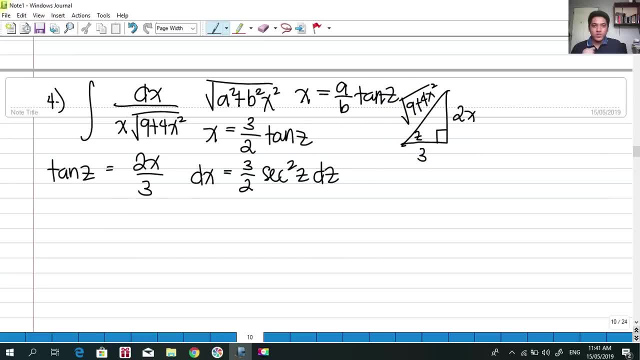 So adjacent over hypotenuse is what Cosine, And hypotenuse over adjacent is secant. Okay, Because 1 over cosine is secant, So we have to use the secant function. So the secant of z is what? 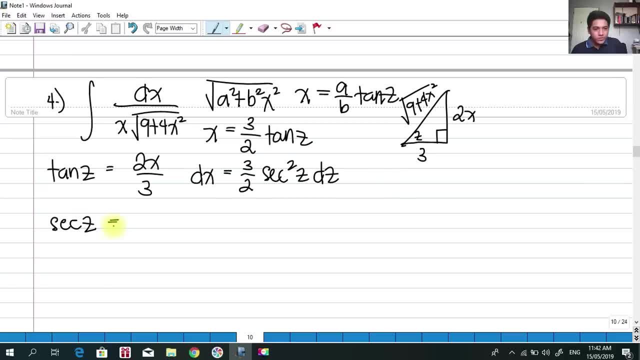 Cosine adjacent over hypotenuse, So secant is hypotenuse over adjacent, 9 plus 4x squared Hypotenuse over adjacent, which is 3.. In order for us to get square root of 9 plus 4x squared, 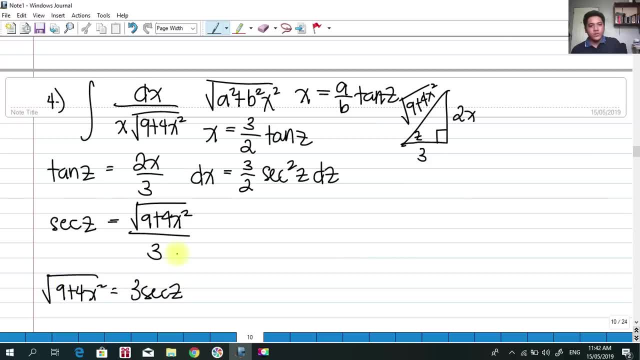 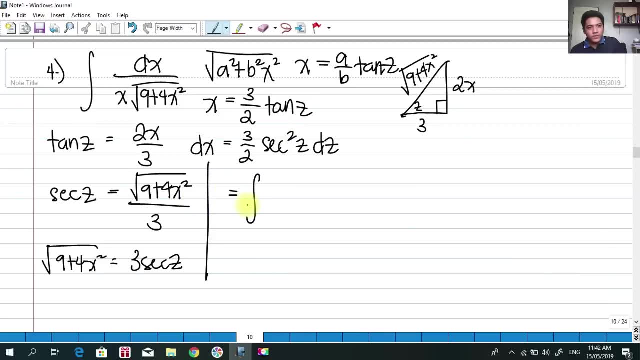 So that is 3 secant of z. So now we can perform our substitution, trigonometric substitution That is equal to integral of dx. The dx is 3 halves secant squared. Secant squared z, d z. Okay. 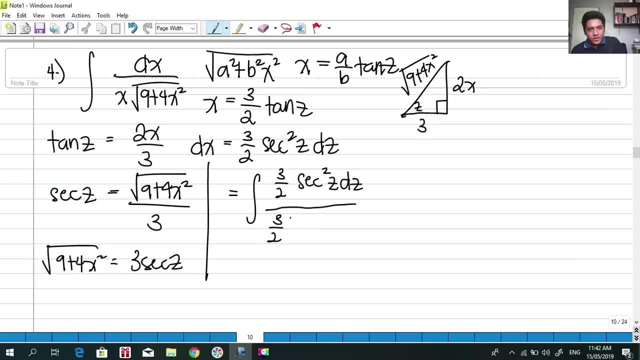 Over dx. what is our x Is 3 halves tangent z. Okay, Multiply it by square root of 9 plus 4x squared, which is 3 secant z, 3 secant of z. So, as you can see, 3 halves will cancel. 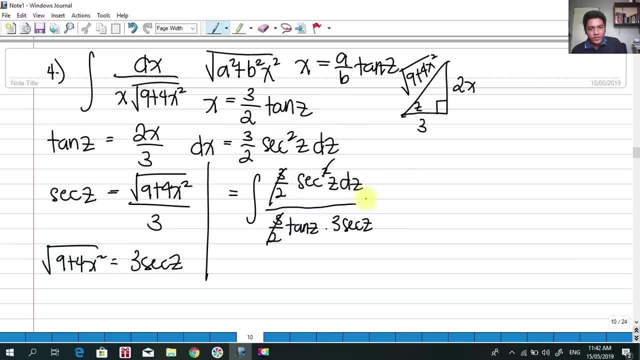 And of course the secant here. one term of secant here will cancel with this, So that you are left with the integral of secant of z d z over what 3 tangent. So we can factor out one-third integral of secant of z d z over tangent z. 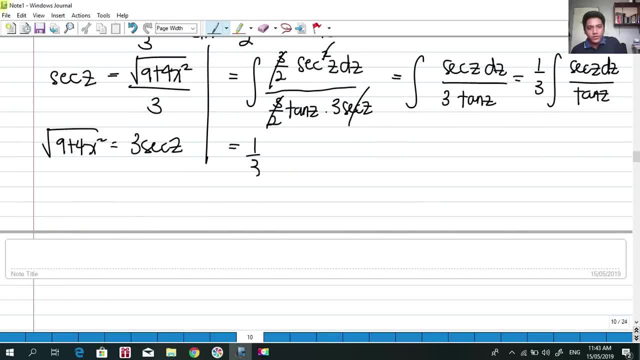 So, again, using some identities, we have now one-third. The integral of 1 over secant is 1 over cosine of z Divided by tangent is sine of z over cosine of z, d z. Okay, And if you are going to cross, multiply or. 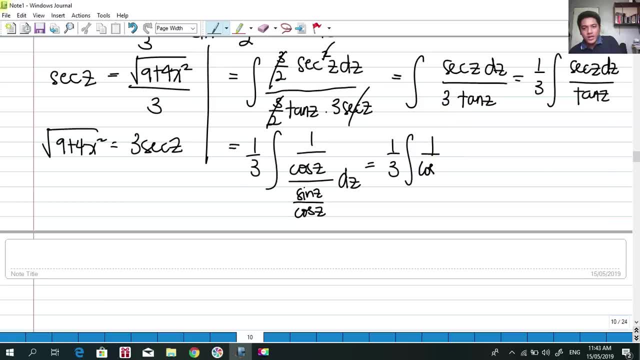 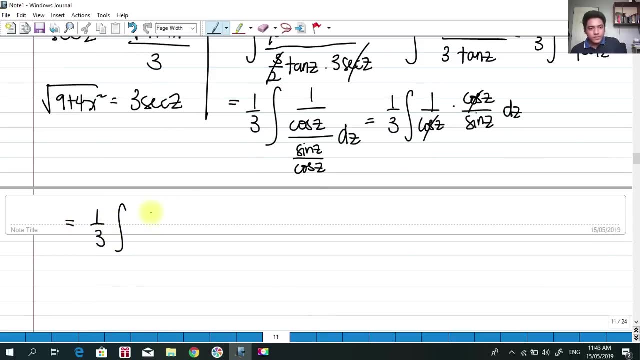 To get the reciprocal and multiply it. So we have 1 over cosine of z, multiplied by cosine of z over sine z d z. So, as you can see, cosine of z will cancel. So we have now what One-third of the integral of 1 over sine of z d z? 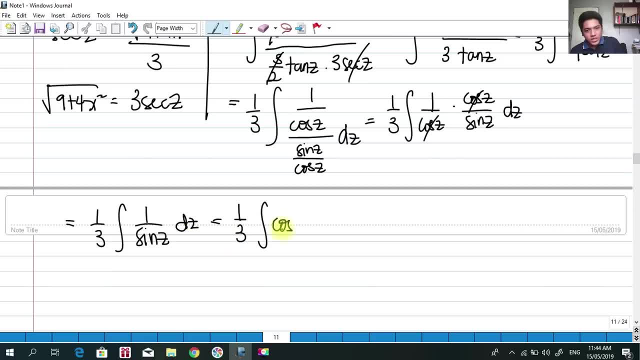 And 1 over sine is cosecant. So cosecant Cosecant of z, Cosecant of z d z. And what will happen is the integral of cosecant is 1-third ln of d. cosecant of z minus. cotangent of z plus c. 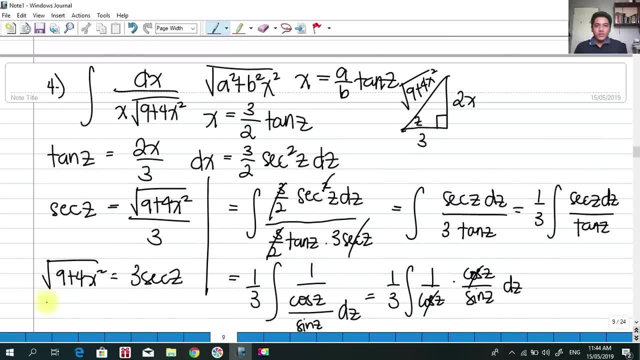 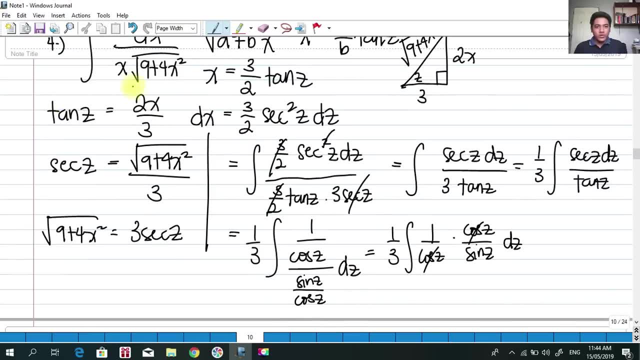 That is not our final answer. We have to get cosecant in terms of this triangle- Okay, And we have to get also the cotangent- Okay, We have the tangent. We're going to simply get d Reciprocal of that. 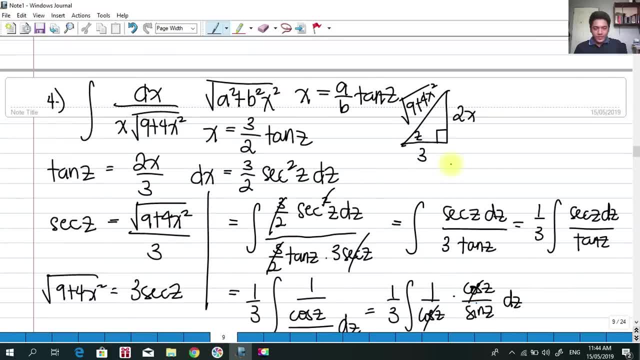 And for cosecant we're going to get the sine Okay Function. So the sine function is opposite over hypotenuse, But its reciprocal is hypotenuse. So cosecant z will now be hypotenuse over opposite. 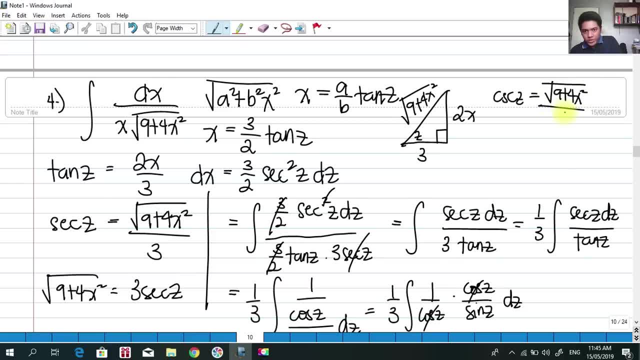 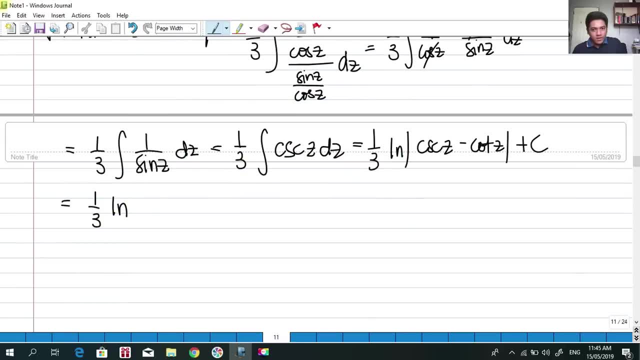 So hypotenuse over opposite, which is 2x. Okay, Cosecant z is that value, So 1-third ln of the absolute value, So 1-third ln of the absolute value of the square root of 9 plus 4x squared over 2x minus. the cotangent of x is simply the reciprocal of the tangent function here. 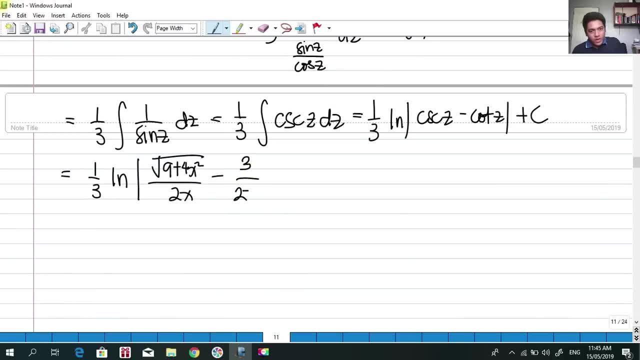 3 over 2x, So 3 over 2x. Absolute value plus c, So 1-third ln of the absolute value of square root of 9 plus 4x squared. Square root of 9 minus 4x squared. 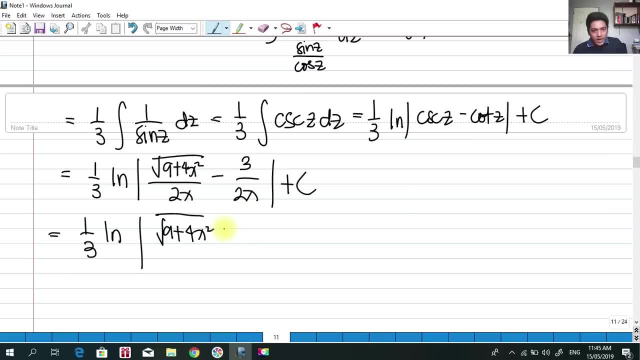 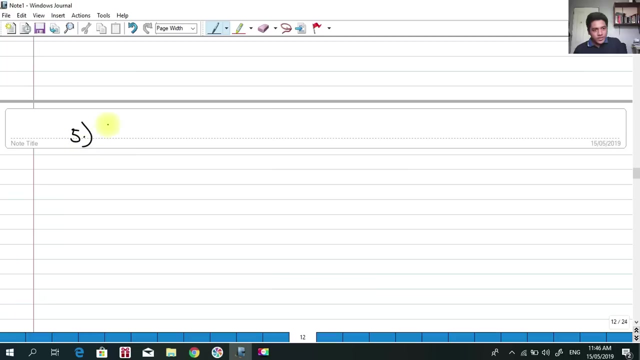 Let me just rewrite Minus 3 over 2x plus c, And this shall be our final answer for the integral. Okay, So down to our last example. This is the last example for this video. 5 is the integral of the square root of 25x squared minus 3.. 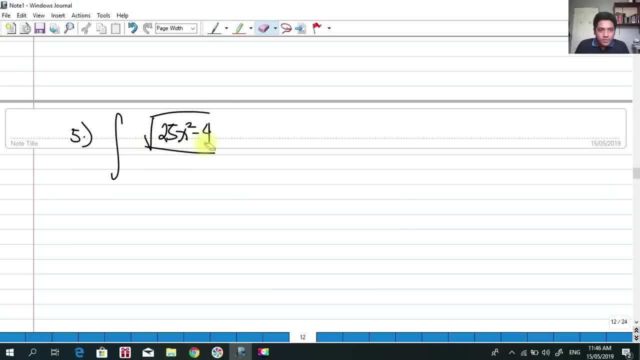 So the integral of 25x squared is 4 over. let me just rewrite over x, dx, x and dx here. So, as you can see, this has a form of the square root of b squared, x squared, minus a squared. 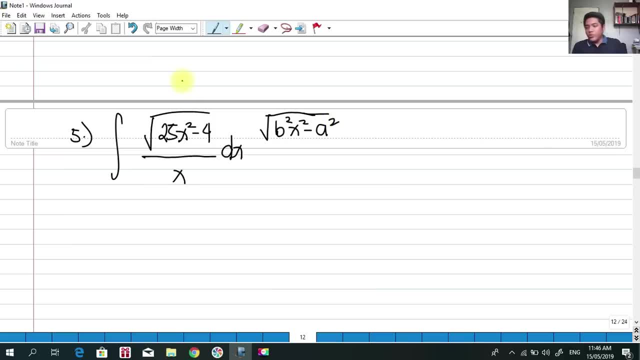 And if we're going to go back to our formula we would be using: x is equal to a over b, secant of z. So, going back to our formula, Okay, If we go back to our formula here, that should be this: 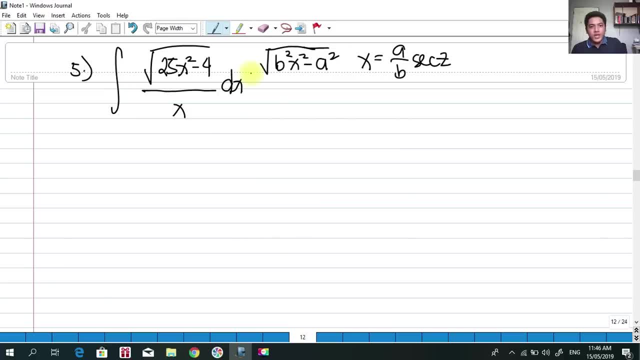 Okay. So again the same process We have. x is equal to our a. here is not 5, but rather the 2 over what 25,? not that, because that is b squared, So the b of that is 5, secant of z. 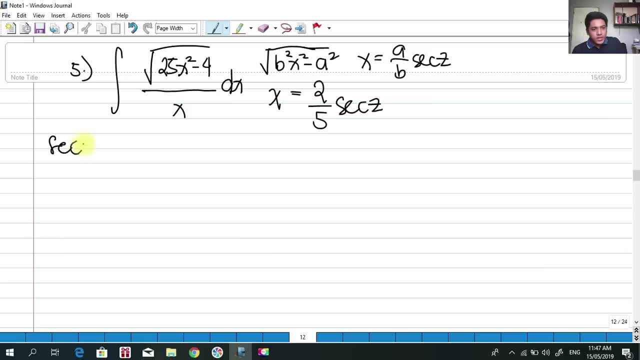 Of course, from that we can derive b, secant of z. Secant of z is 5x over 2.. And from that we can derive our right triangle. Okay, This is our side z, or the angle z. So secant is the opposite of cosine, wherein cosine is adjacent over hypotenuse. 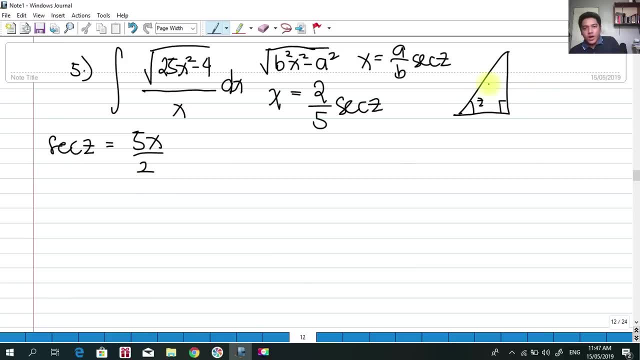 So this should be hypotenuse over adjacent. So our hypotenuse is 5x, Adjacent side is 2.. And therefore this must be 25x squared Minus 4 divided by Pythagorean theorem. 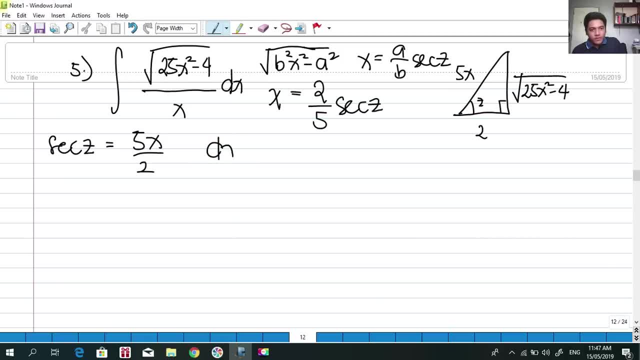 And what are we going to do again is to get the derivative of x here And the derivative of this 2 fifths secant of z, tangent z, bz, And of course we're going to get this term, this term, okay. 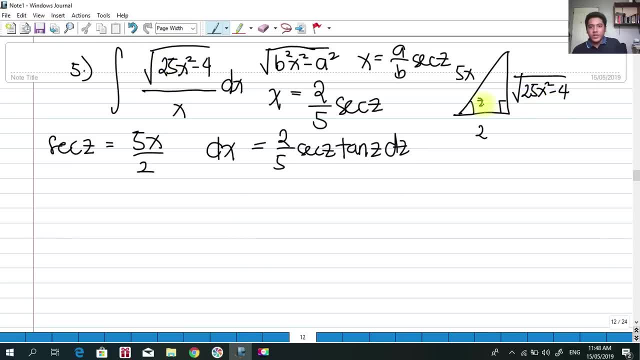 Square root of 25x squared minus 4 using our triangle. So, as you can see, here we cannot use hypotenuse because it has a term x, So it's much easier. We don't want to use that, So we can only use adjacent and opposite. 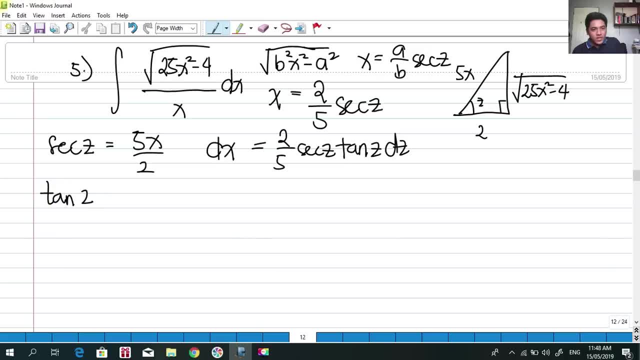 So we can use the tangent function. Tangent of z is opposite over adjacent. Okay, Tau, 1. Opposite is square root of 25x squared minus 4 over 2. Cross multiplying we have square root of 25x squared minus 4 is equal to 2.. 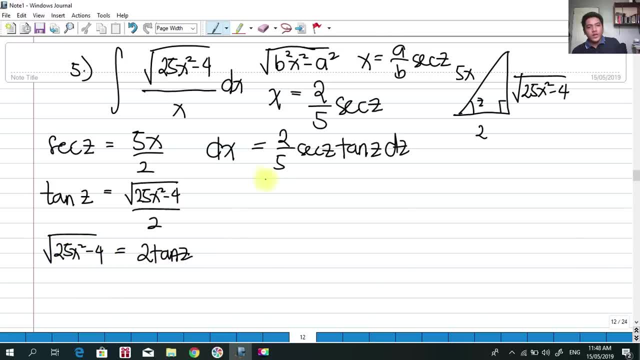 2 tangent of z. Okay, And therefore we can now solve our integral So that integral is equal to square root of x. squared minus 4 is simply equal to 2 tangent of z over x, which is here 2 fifths of secant of z multiplied by dx. 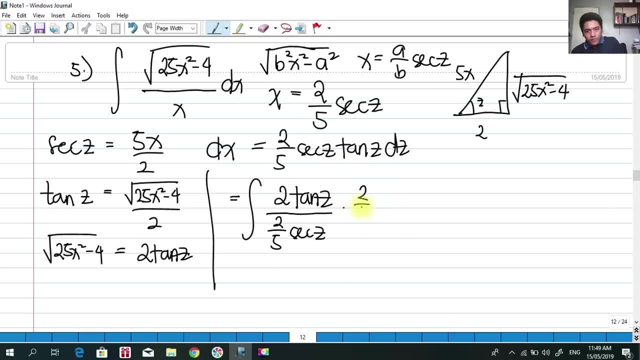 Our dx is 2 fifths secant of z, Tangent Z, D is a. So, as you can see here, 2 fifths will cancel as well as the secant. Okay, Then we are left with what? 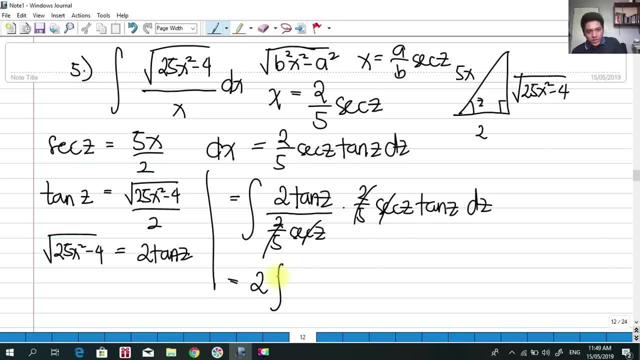 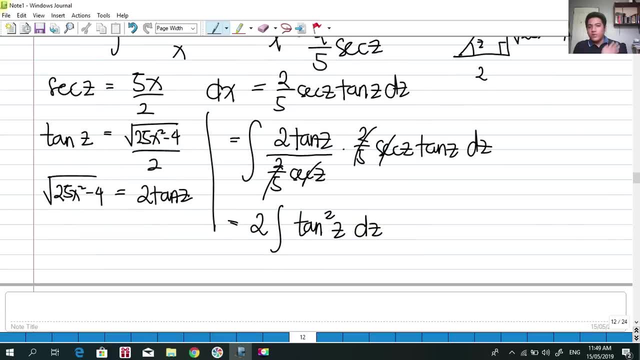 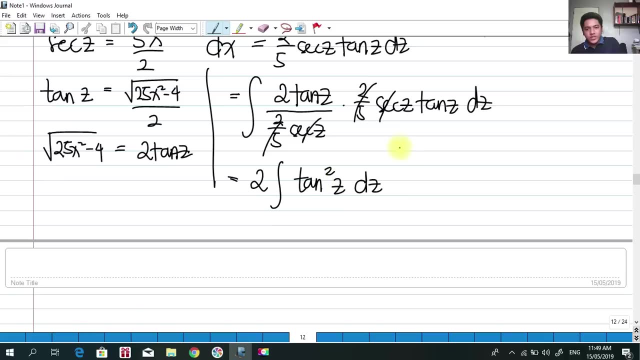 2. tangent z times tangent z is- We can factor out 2, the integral of tangent squared z D is a, So we can. what We can actually transpose or transform this Tangent squared z Into secant squared z minus 1 is equal to tangent squared z. for us to integrate this. 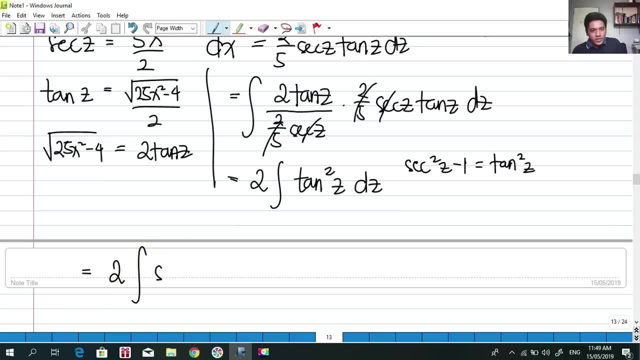 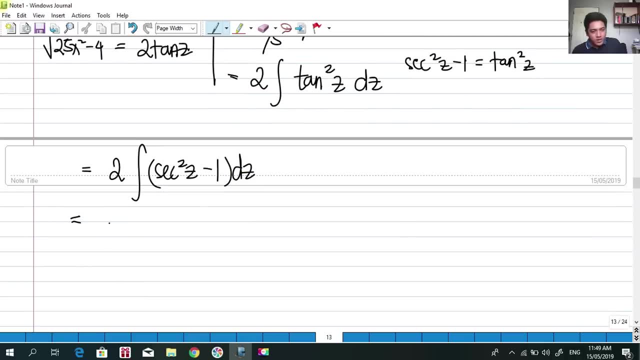 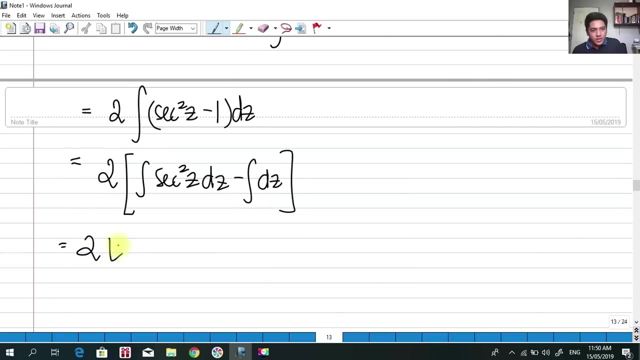 So we have 2 integral of secant squared z minus 1 times dz. Well, of course, we can integrate this independently. So integral of secant squared z, dz minus dz, simply Okay. So integrating that We have 2 integral of secant squared is tangent of z minus integral of dz is simply z plus c. 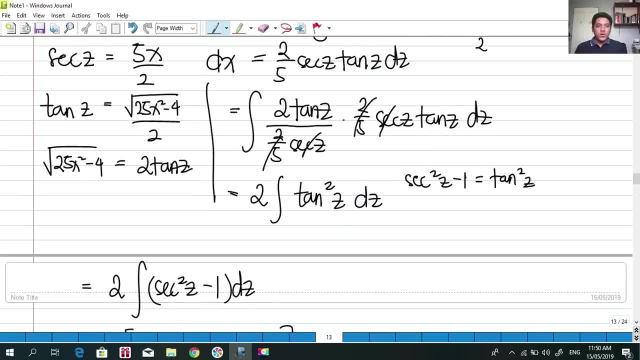 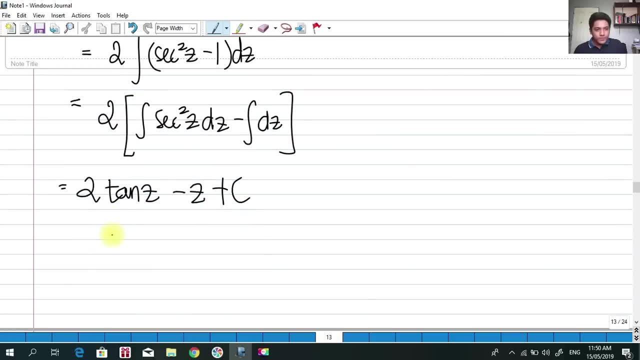 Right And going back, let's substitute this z into x, So our tangent z is equal to square root of 25x squared minus 4 over 2.. So we have 2.. What 2 times square root of 25x squared minus 4 over. 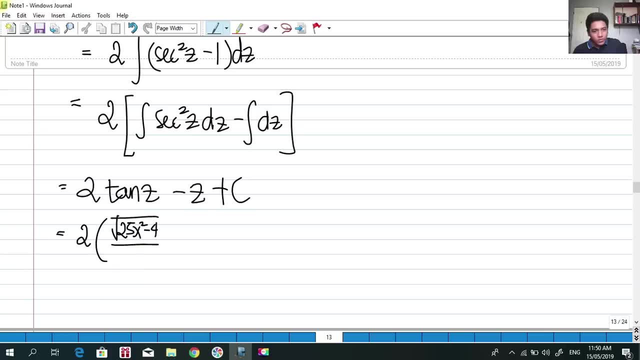 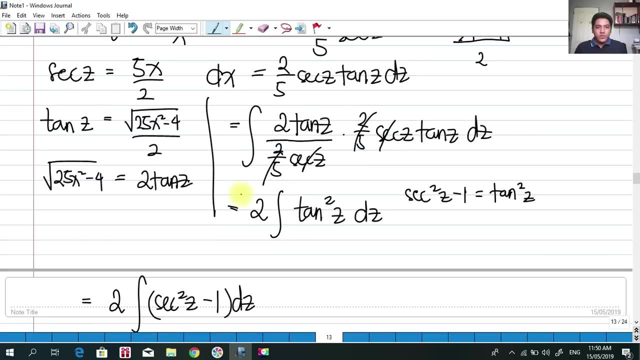 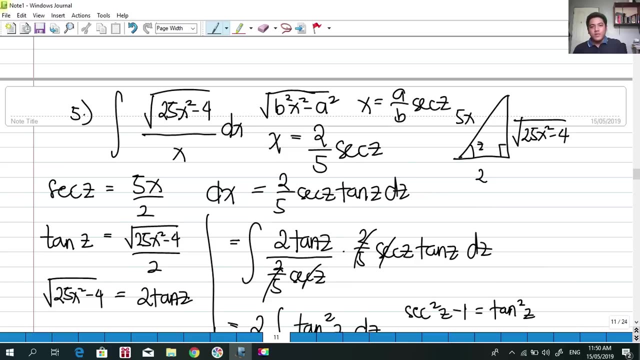 Is that 2?? Is that 2?? Is that 2?? Yes, That is 2.. Okay, 2.. And these 2s will cancel minus z. We don't know the z. Okay, So we can, based on the choices, we can pick the z as the. we can get the z by this trigonometric. 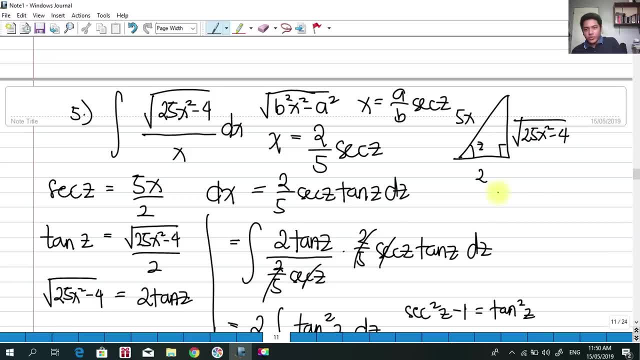 function. Okay, Based on the choices. So in this case I'm going to use cosine of z. Cosine of z is k. Okay, Adjacent over what? Adjacent over hypotenuse? So 2 over 5x. 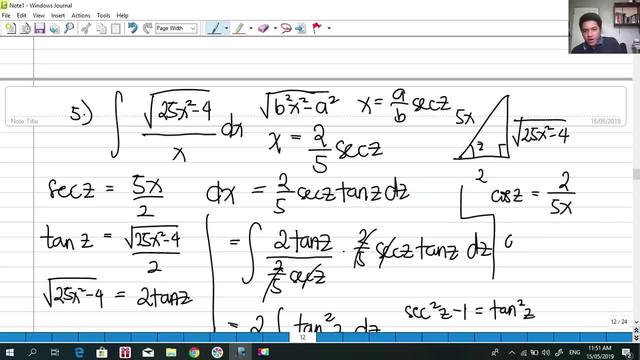 Okay. So rearranging this, we can get r, We can get z. We can get z by what? Okay, z is r cosine of 2 over 5x And that should be our z. Okay, So z is r cosine of 2 over 5x. 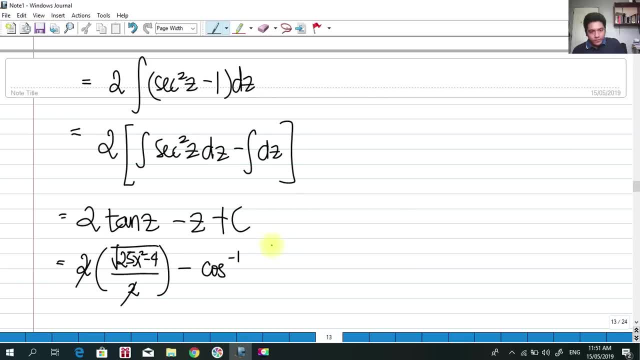 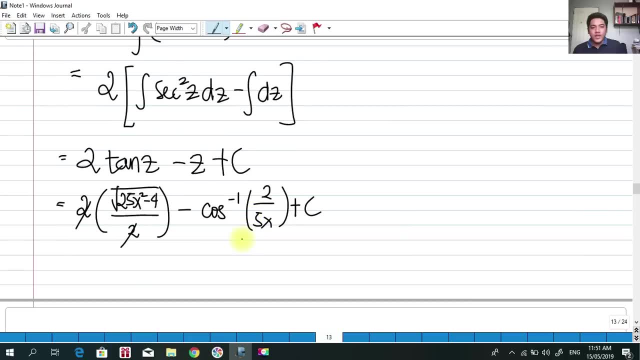 So r cosine of 2 over 5x plus z, And again you can get the z in different trigonometric functions based on the choices, But of course I only use the cosine function, So you are not limited to do that. 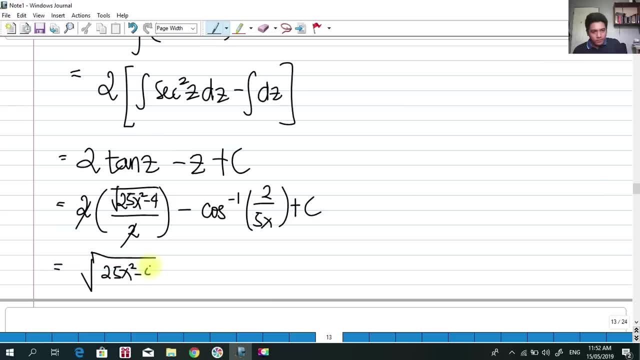 You can use tangent or whatsoever you want. Okay, So this would be resulting into square root of 25x squared minus 4, minus the r, cosine of 2 over 5x plus z, And of course, okay, Of course we forgot to distribute 2 here. 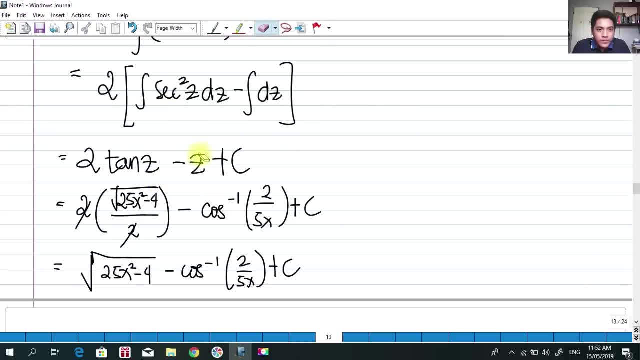 So this should have also a 2.. Okay, I'm sorry. So we have negative 2z here, So this should have a 2, because, again, we try to distribute this 2.. So this should have a 2 here and here. 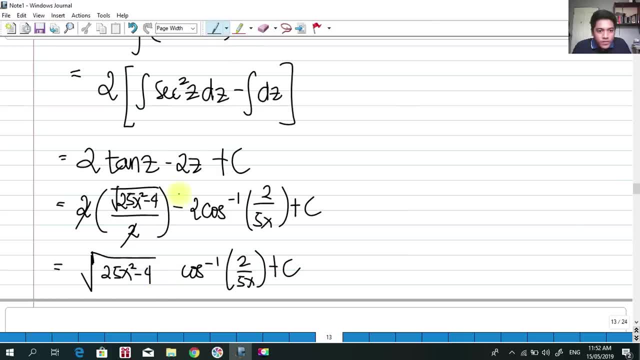 So our final answer would be: square root of 25x squared minus 4.. Okay, Minus 2.. Okay, Minus 2, r, cosine of 2 over 5x plus z. Okay, And again we distribute z.